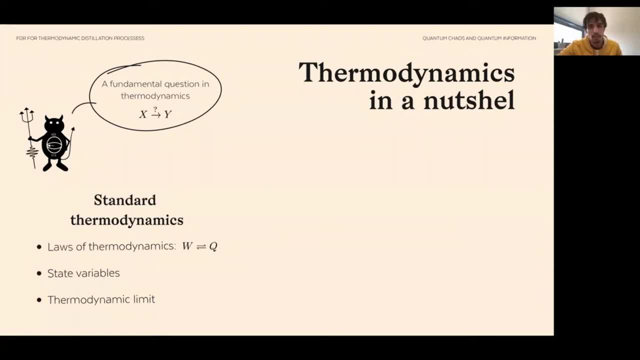 do under thermodynamics- classical thermodynamics- and I usually do under thermodynamics, classical thermodynamics- In a limit called thermodynamic limit. what does it mean? It means that my system is composed by some number of particles, and this number of particles tends to infinity. 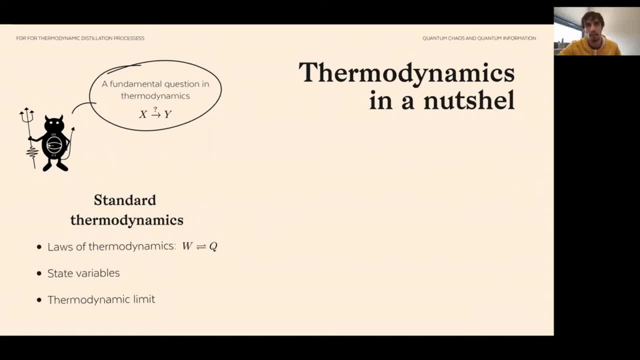 And also that all the processes are taken very slowly in the quasi-static regime, because I have always to keep the equilibrium okay. And then the question. and then, for example, I can imagine that my system is, I guess, inside of a chamber and the states where 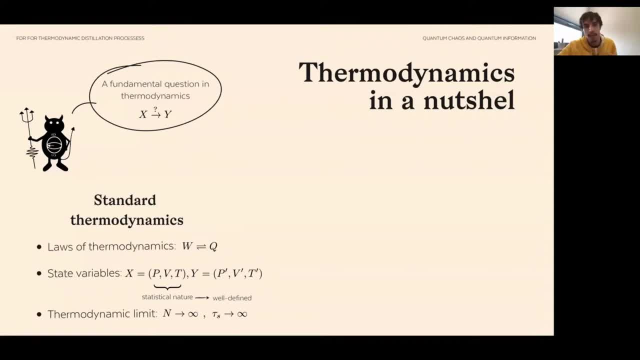 able will be pressure, volume and temperature, And although they are statistical by nature, they are well-defined because we are in this limit in which n tends to infinity. These quantities are average and fluctuations in this regime doesn't play any role. 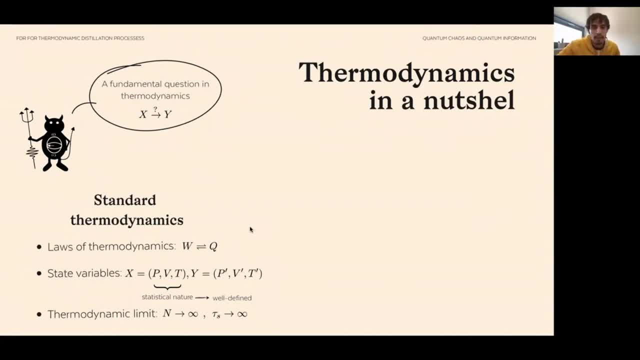 So the question is, the natural question is: what happens if I go beyond the thermodynamic limit? What does it mean to go beyond? It means that I don't want to look to a system in which the number of particles tends to infinity, but I want to look for a system. 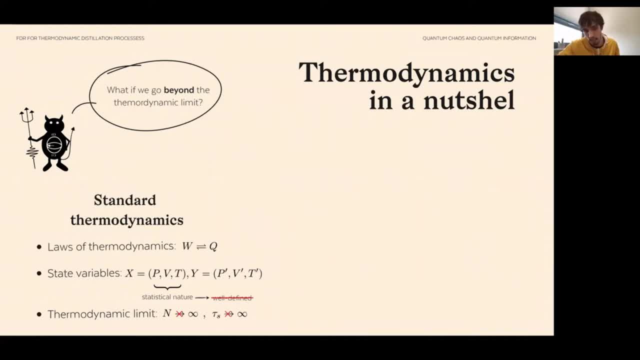 which is composed by a finite number of particles, for example. Well, what we can see is that my state variables. it won't be well-defined anymore because fluctuations will play a role, because I'm far from this thermodynamic limit. So I need. 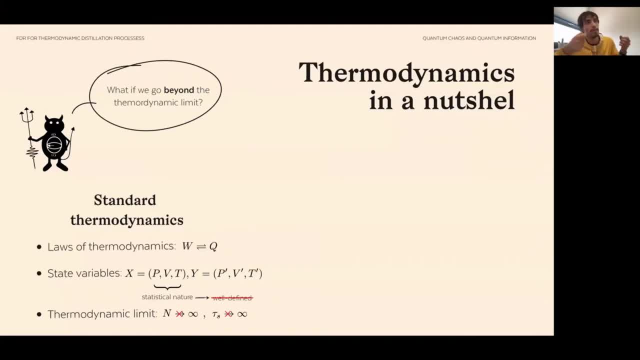 a new set of components, So I need a new set of constraints if I want to think about what is the constraints associated with states transformation. So for example- just a motivated example- we can think that I want to extract work from n subsistence And we know that by applying 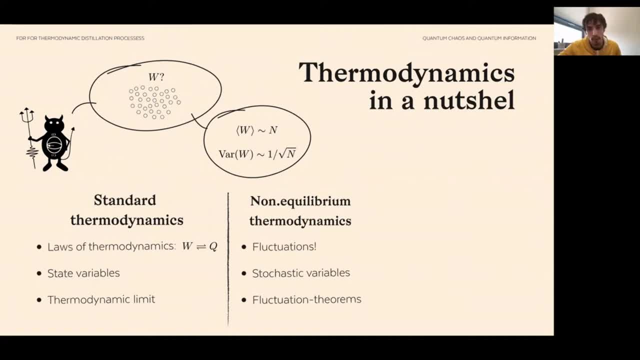 the central limit theorem, the average of work scales with n, while the fluctuations associated to the work will scale with the inverse of n. Okay, The inverse of the square root of n. In other words, fluctuations will play a role. So what I can do is: let's imagine that now I'm going to treat these thermodynamic quantities. 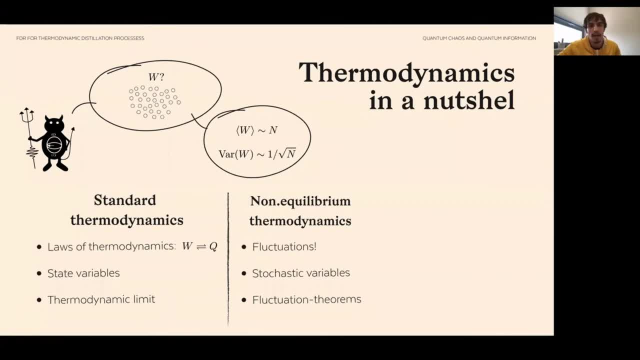 for example work, heat and entropy as stochastic variables. But again, thermodynamic will give me more restrictions because these stochastic variables will be described by some probability distribution function. So for example some probability distribution function of the work. but these probability distributions they cannot be arbitrarily. 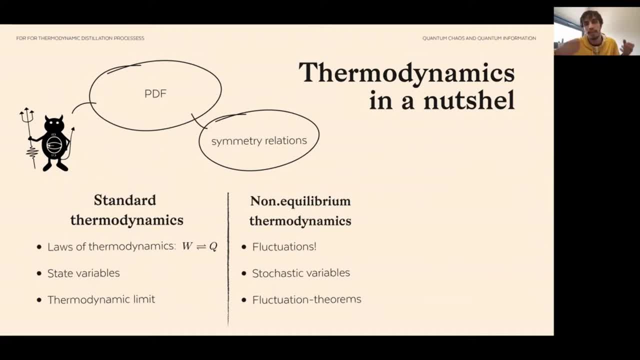 ones They most respect, some relations called by symmetry relations, And the symmetry relations is a collection of theorems called by fluctuation theorems. A very famous example of fluctuation theorems is the Jerezinsk equality, which allow us to express inequality from the second. 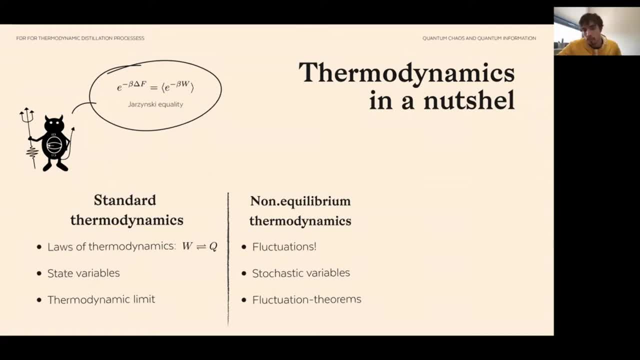 law as equality. And just to Now let's go back to the three-dimensional model. Here I'm going to make sure in this we are in the non-equilibrium regime, Okay. So since in this regime fluctuations play a whole, we need a new set of tools to describe this system. And then another question is: 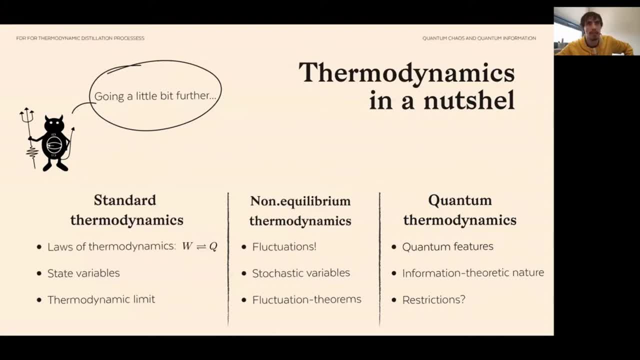 what happens if we go a little bit further? What does it mean? if I look to systems even even smaller, Such that now I Not only thermal fluctuations will play a whole, but also thermal fluctuations will play a whole, also quantum ones. 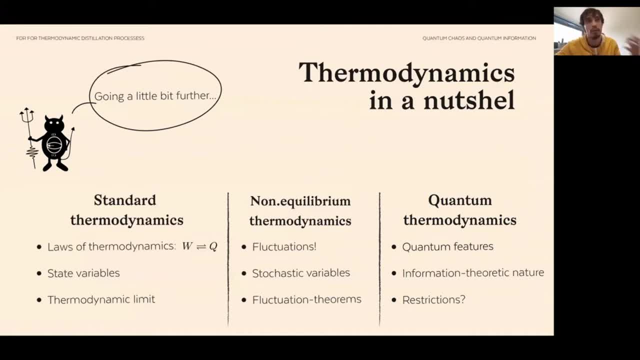 Are you being a scenario in which I have the presence of quantum features And then I can ask this question again: how thermodynamics, quantities can be carried over to the quantum helm? What is the constraints underlining states, transformations? One of the things that I can tell you. 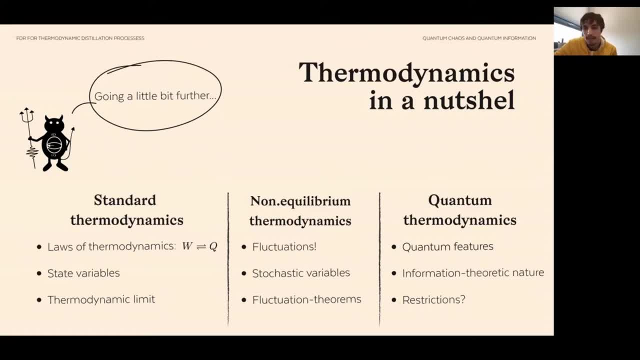 I spoiler about my presentation is that in this regime, not only fluctuations plays a whole, but also information. Information is a very meaningful quantity in this regime because the thermodynamic quantities- I will show you these- can be expressed in terms of informational quantities. 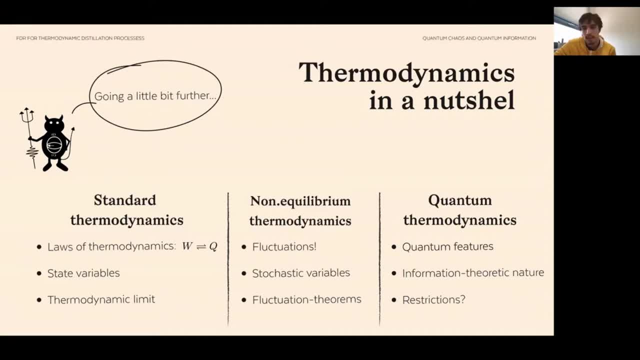 So with these, I can again ask the question that I started this transference, which is what states transformation are thermodynamically allow it for a given state in this regime? Well, when you see that, there is the results that I'm gonna show you. 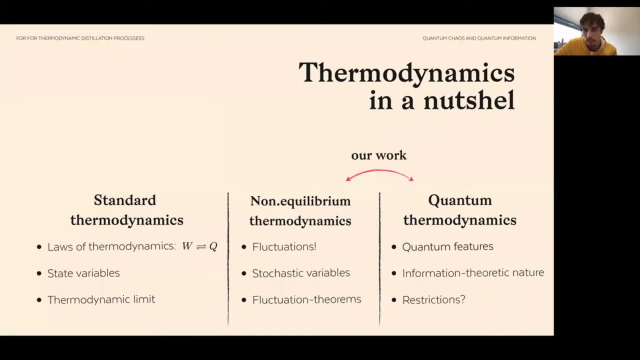 I'm gonna show you today comprehends these two scales will be between this intermediate regime, between classical and non-classical, And the way that I'm gonna address this question about states transformation is by looking for how I can manipulate some resources, under free operations, for example. 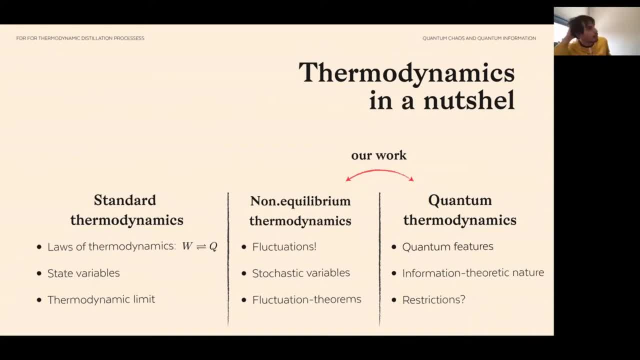 And because, if I think that thermodynamics is a theory of restriction, we know a mathematical framework to deal with these restrictions, which is the resource theory framework. So this question can be translated into a study in which I study how I will manipulate resources under operations that I can do it for free. 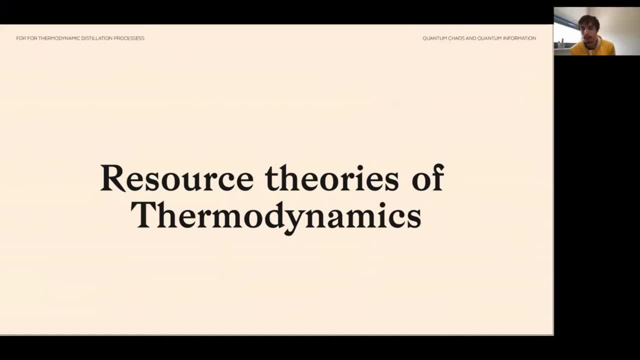 So let me start telling you about the building block, The building block of our framework, which is the resource theory of thermodynamics. But first let me remind you very roughly that a resource theory is defined by three ingredients. First, the set of free states. 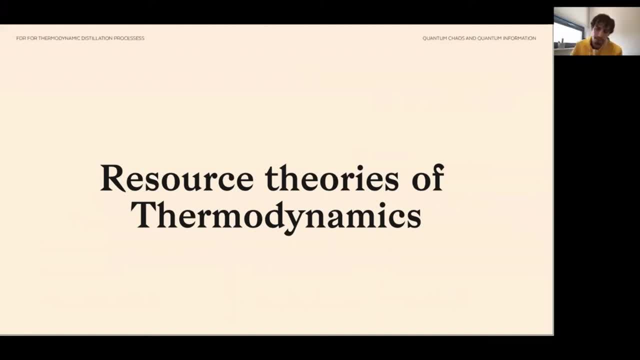 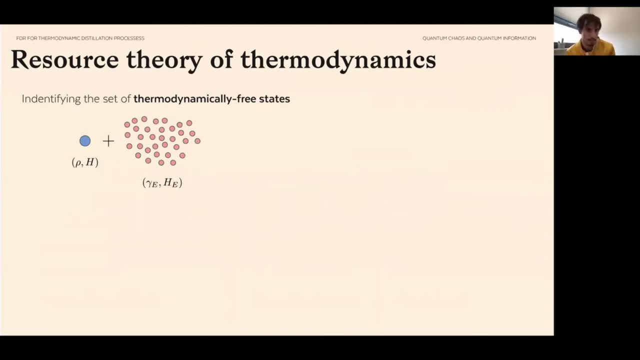 the set of free operations and the monotones. In our case, in my whole presentation we will see this scenario With scenario. I have a system here represented by this blue circle. The system is described by some state row and some Hamiltonian age. 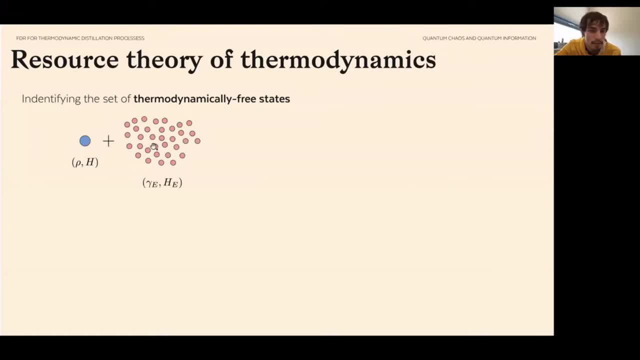 And this system is interacting with a thermal bath at inverse temperature beta. The thermal bath is described by a thermal distribution, here denoted by gamma and Hamiltonian age E. okay, Well, we know that if I take my system, couple with the bath and let my system to relax. 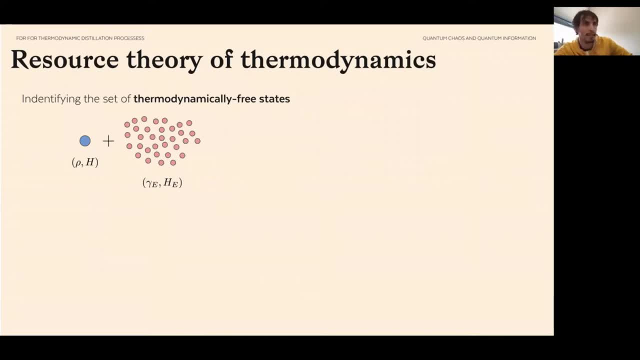 in the asymptotic limit in which the time tends to infinity, my system will be termalized. In other words, if I have system and bath, I can always achieve the thermal equilibrium. So a free state of my theory is a Gibbs state. 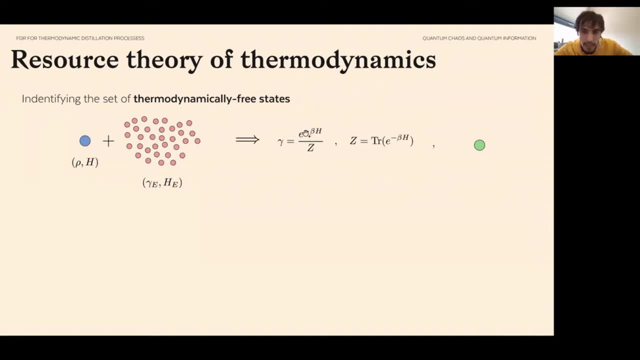 is a thermal state, which is denoted by this expression here. such this beta here is the inverse temperature of the bath and Z is the partition function, defined like this. In other words, every state which is not thermal is a resource state. Every state which is out of equilibrium is a resource state. 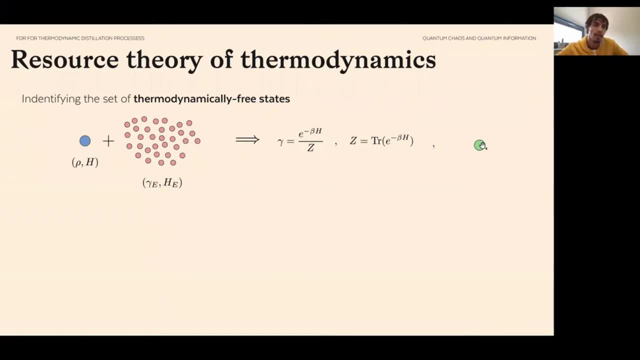 So, for example, this green ball here. So I'm using this funny notation, for if the state is not red, it's not red balls, it's a state out of equilibrium, but it's red. or if it is red, it's thermal equilibrium. 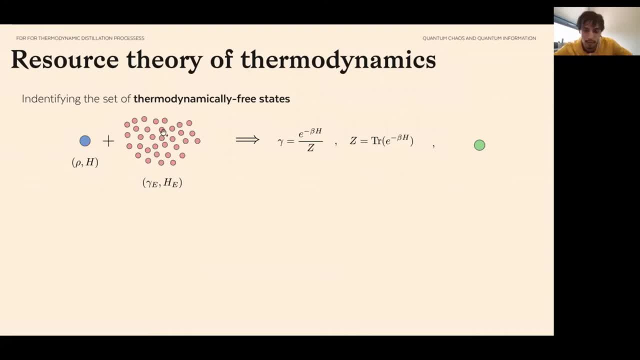 If you have a collections of small balls, you have a thermal bath. This is just to make it more simpler, okay, And then what about the set of three operations? Well, three operations of my resource theory will be modelled by thermal operations. 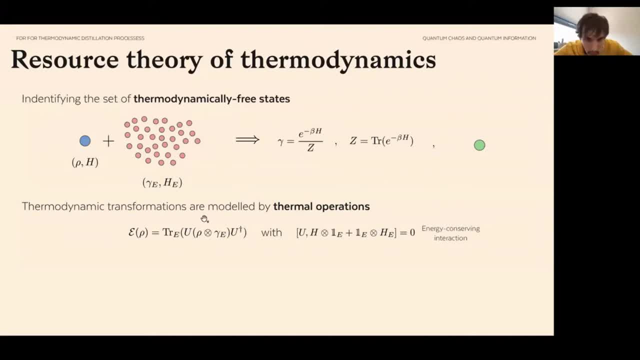 Thermal operations are C-P-T-P maps defined as follows: So basically the idea is that I have my system, I will couple my system with the thermal bath. I will involve both under this joint unitary. here This unitary is called energy conserving interaction, because 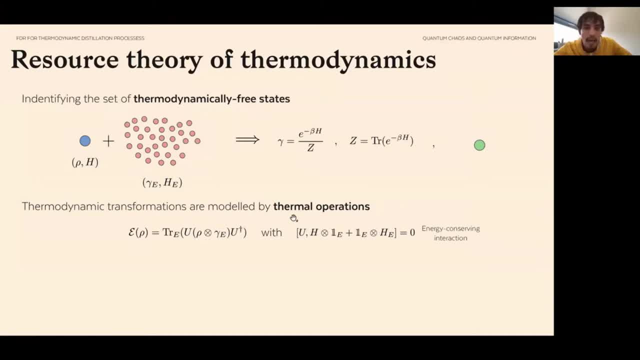 it commutes m Hamiltonian of the system and the Hamiltonian of the bath, And thermal operations are free because thermal operations encodes the first and the second law of thermodynamics, because they satisfies two properties. The first property is that the thermal state 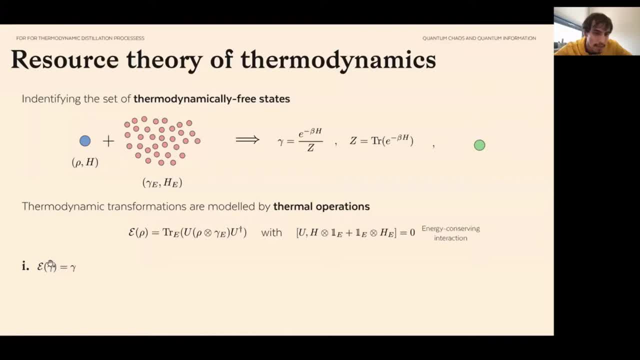 it's a fixed point, which means that if my state is given by a Gibbs state and I apply a thermal operation, I must return to the thermal state. Otherwise I would be creating research and I would be violating the second law of thermodynamics. 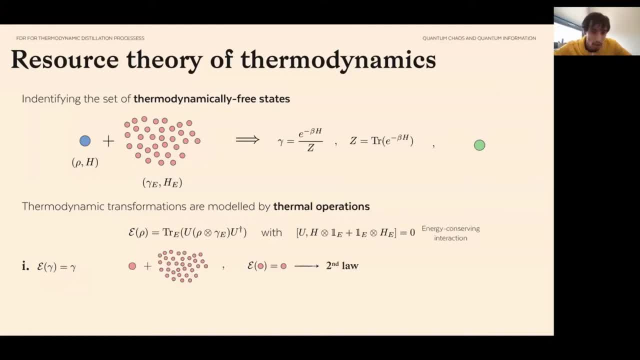 Let me be more explicitly in explaining this. So let's imagine that I have a thermal state, this red ball I couple with the bath, I involve both under this big unitary here and I have to return. I have to get a thermal state in the end. 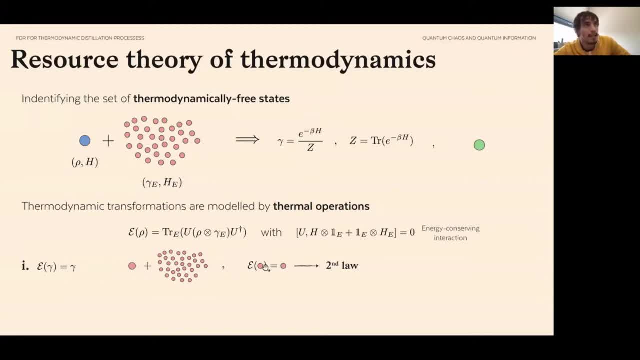 If not, imagine that the result of this is a state out of equilibrium. I could take this system out of equilibrium couples with the bath again- let it relax- and doing this equilibration process- I'm striking work And then I could repeat the same process. 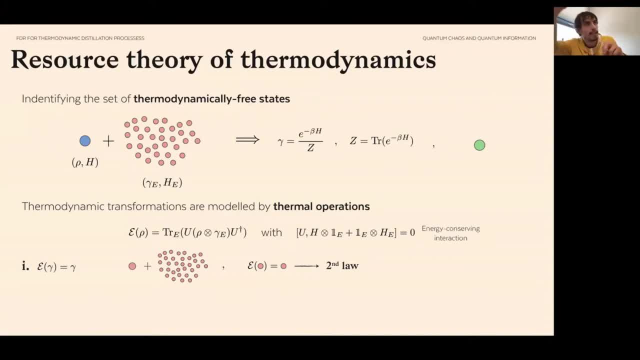 I could apply some thermal operation, take the system out of equilibrium and relax again, And by doing this I'm creating a perpetual mobile, or in other words, I'm violating the second law of thermodynamics. So we say that this first property 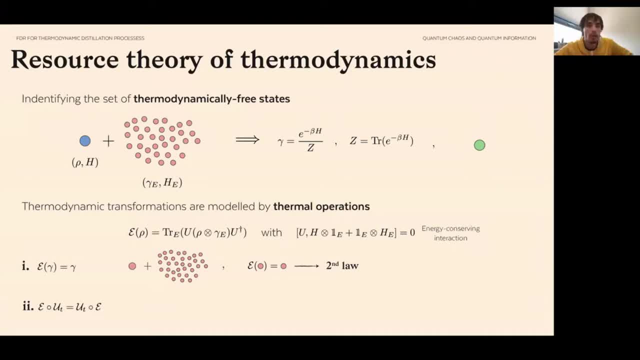 encodes the second law of thermodynamics. The second property tells us that thermal operations are time translation covariant. What does it mean? It means that it doesn't matter if you first let's say that you have system and environment, If you first involve system and environment. 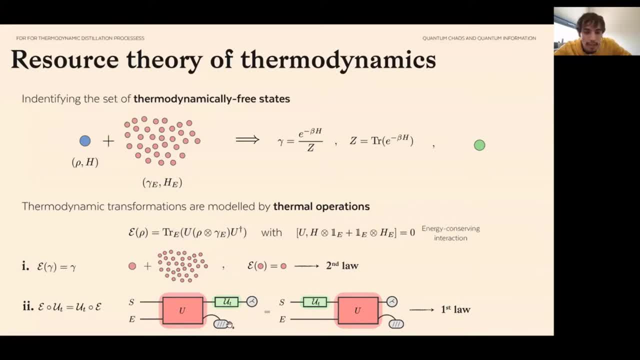 via this big unitary, you trace out the system and then you involve system on time and measure the time. This is the same as involving the system first on time, then involving, via this big unitary here, Tracing out the bath and then measure the system. So in other words, these, these properties telling us that energy has been conserved. So the first law of thermodynamics is encoded in the second property. 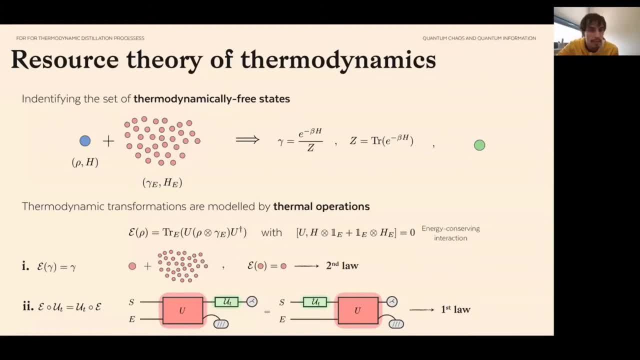 Okay, so basically here I have my two ingredients: the set of free operations at the set of free states and the set of free operations. And now my last ingredient. to My last ingredient is the definition of monotone. So a thermodynamic monotone is a function that map the set of quantum states into positive real numbers, with the inclusion of the zero. 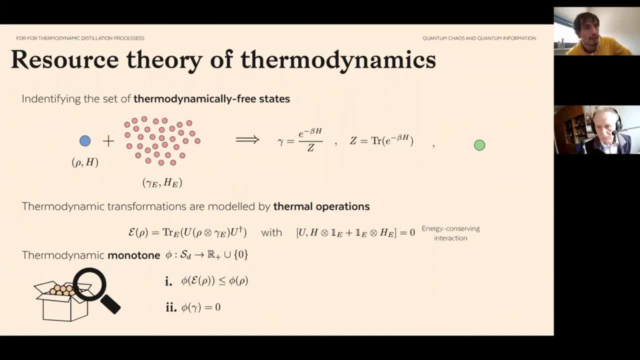 And a thermodynamic monotone quantifies the amount of resource that a given system has. So, for example, to be a monotone, this function has to satisfy these two properties. The first property tells us that monotones are decreasing energy. The second property tells us that monotones are decreasing under thermal operations. 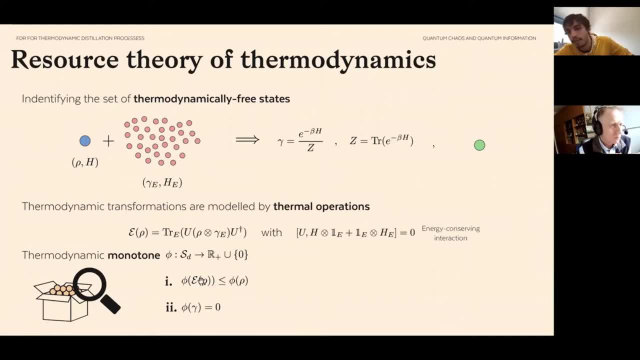 And this has to be to be satisfied, Otherwise, by thermal operations I'm creating resource, and we know that if I create resource, I'm violating the second law of thermodynamics. And the second property tells us that thermal states don't possess any kind of resource. So the monotone assigned to thermal state gives me zero. 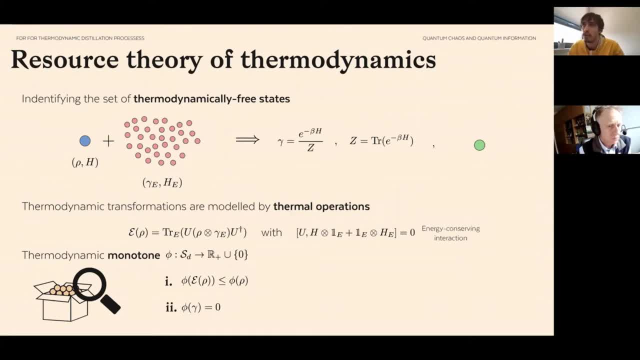 So, okay, As I've been mentioning resource, resource, and by resource I mean states out of equilibrium. Okay, Perfect. An example of thermodynamic monotone is the relative entropy between rho and a thermal state. This quantity here is defined as follows. 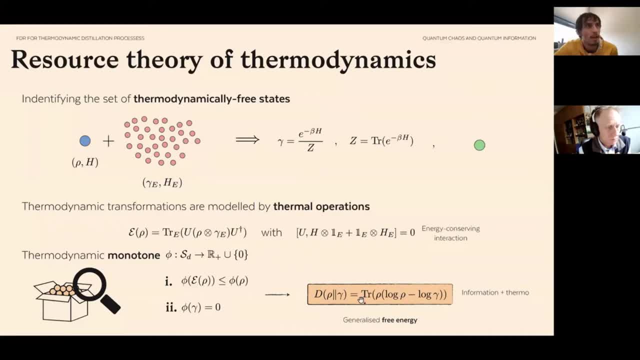 And this quantity has some kind of. This is the first time that we see a thermodynamic quantity being expressed in terms of a informational quantity, Because what you see in the next slide that this quantity here called by non-equilibrium free energy. it's a generalization of the concept of free energy. 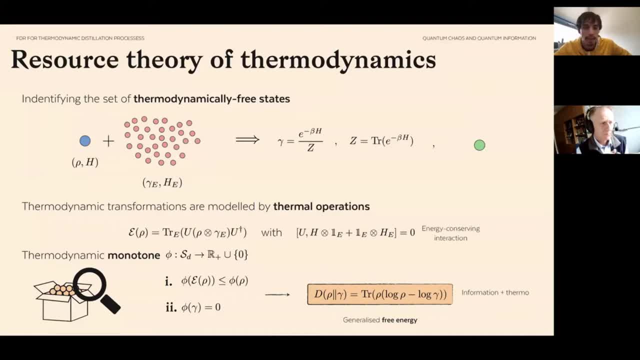 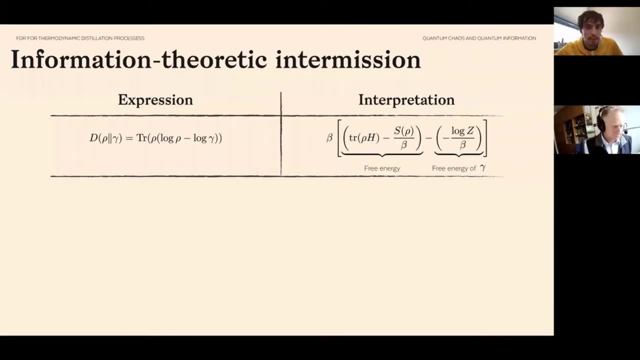 And this quantity tells us how much work, what is the maximum work that you can extract from a system which is out? We already saw a connection between informational quantity with thermodynamic quantity. Let me show you some other Thermodynamic quantities which will be expressed in terms of informational quantity. 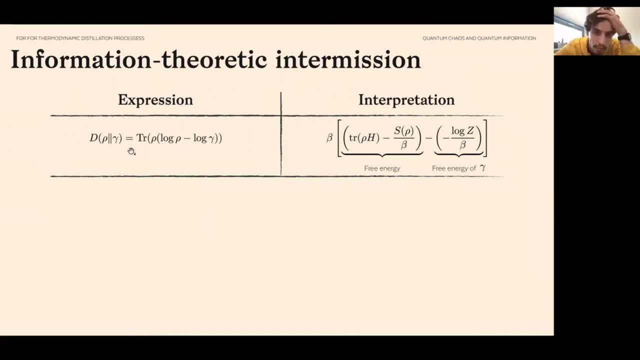 So, for example, I already mentioned the non-equilibrium free energy, And since this expression is the general one, I'm going to call it by, only by free energy And the free energy. if I, for example, open this term, what does it mean? 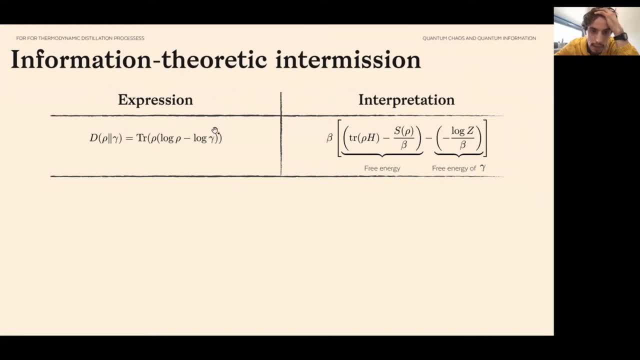 It means that if I substitute here E to minus beta H over Z, I'm going to get this expression here, And from this expression we can see why the relative entropy between a given state and the thermal state is called as a generalization of the concept of the free energy. 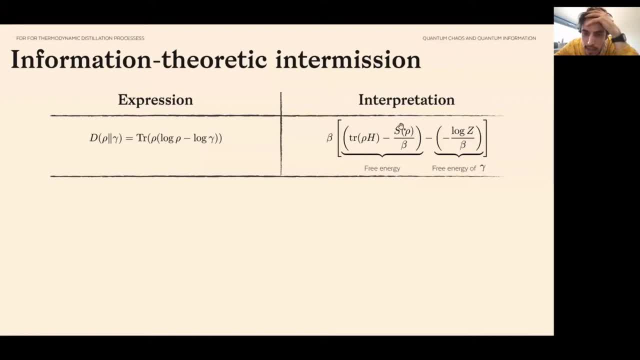 Because, look that the first term is basically the free energy associated to your state, While the second term is the free energy associated to the thermal state. And if we remember about classical thermodynamics, the maximum amount of work that you can extract from a given system is given by a free energy difference. 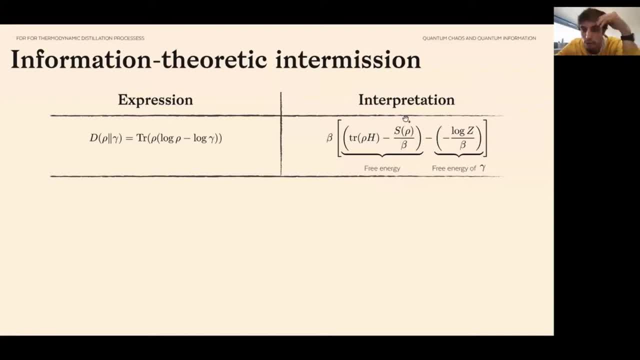 So here I have a free energy difference, But so this quantifies the maximum amount of work that you can extract from a system which is out of equilibrium. But let me point it out that this entropy which appears here is the von Neumann entropy. 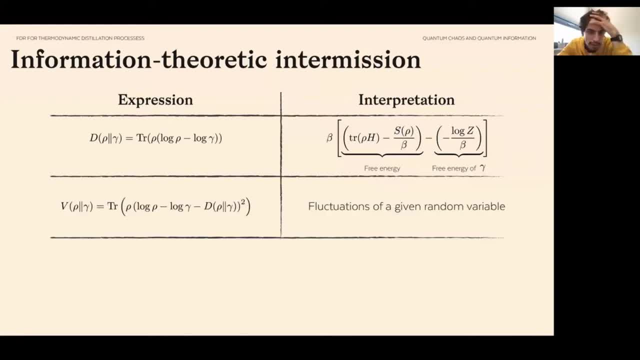 OK. So the second quantity, the second, the second informational quantity, which you have some thermodynamic interpretation, is the relative entropy variance. It is a quantity defined like this, OK, And this quantity tells me some about some fluctuations of a given random variable. 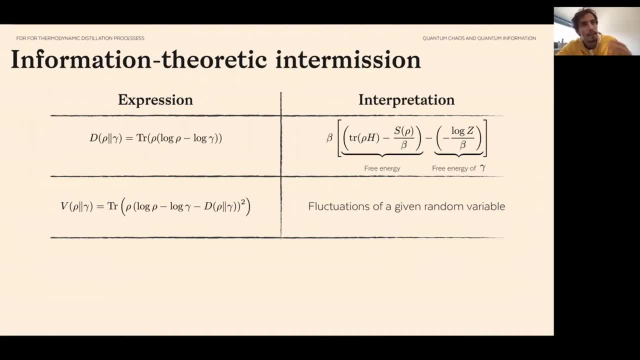 So in the seminar, we in the seminar, these fluctuations will be free energy fluctuations. But if they, if the initial state here is pure state, these fluctuations becomes only energy Fluctuations. And if we're computing, this function between two thermal states. 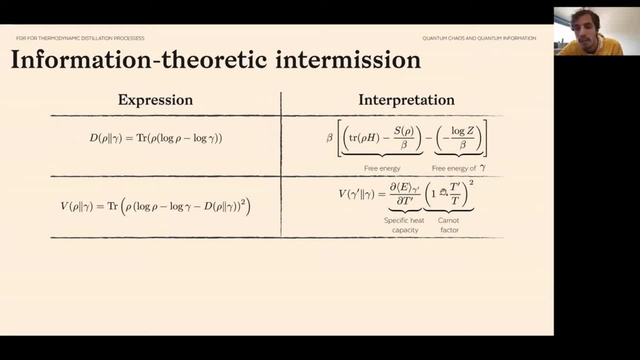 but with different temperatures, you have a quantity which is proportional to the heat capacity. The last informational quantity that I want to introduce is the relative entropy skewness, which is an expression defined like this, And this expression is a little bit tricky to interpret. 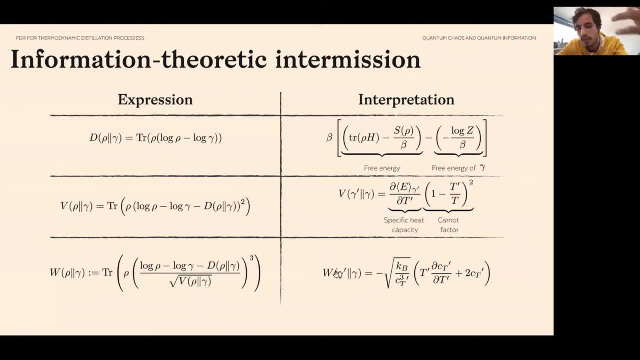 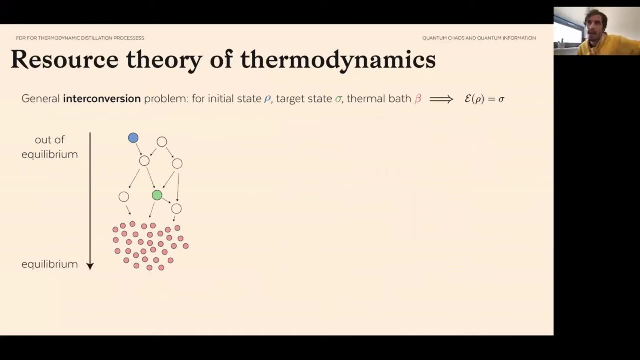 But it's interpretation is that this, this, this function is this quantity is a function of the derivative of the heat capacity with respect to the temperature. So, since we have the tools that I wanted to present to you, let me introduce you to now to the question that I'm interested. 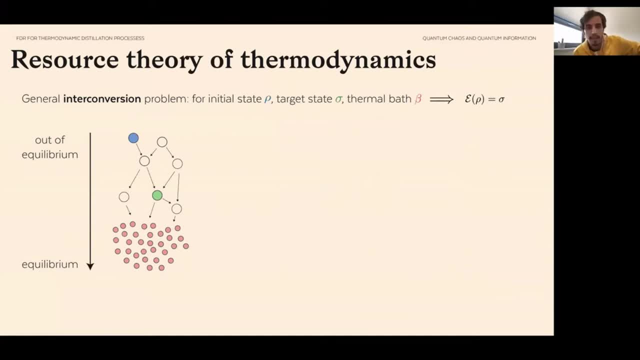 But let's start from the basic. Let me start by saying about the general problem, The general problem in resource theory of thermodynamics, not specifically to resource theory of thermodynamics, but here the problem that we are interested. So the so. so this problem is called the general interconversion problem. 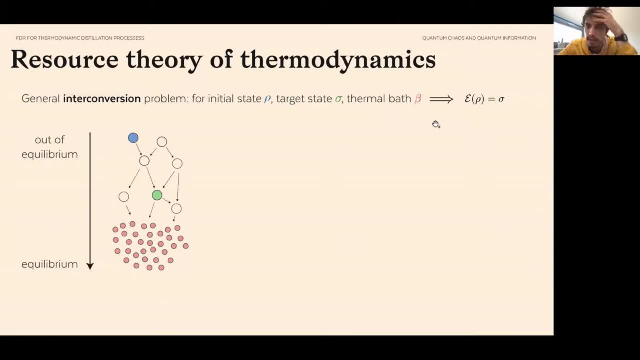 And this problem consists in asking whether there exists some thermal operation, mapping, some initial state rule to some start, to some target state sigma. Why? Why You have, Why You are able to use the bath. So, for example, you have some initial state. 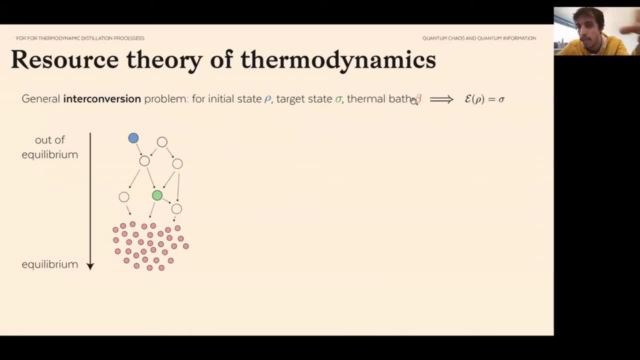 You have your target state and the thermal bath at inverse temperature, beta, And you ask whether you can transform a row to sigma via thermal operations. So in this, in this picture here in the left corner, it's a very nice illustration about this problem. 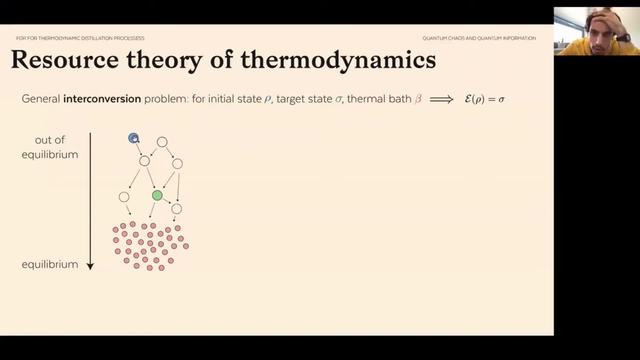 because let's imagine that my initial state is this blue ball, My, my target state is this green ball, And then we can ask whether we can go from this blue state to the target state. And you know, you see this arrow pointed to out of equilibrium states, to equilibrium, to. 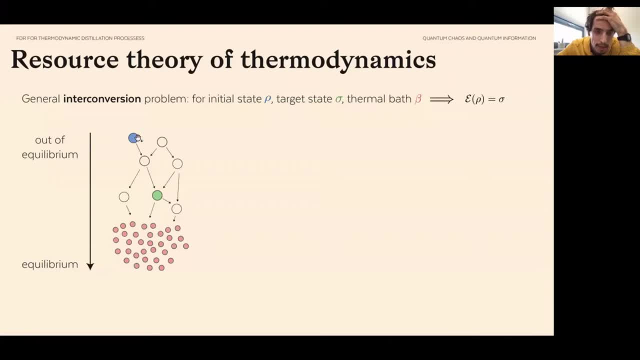 equilibrium states. Why? Because every time that you make a transition, you are dissipating some amount of resource. Okay, You are basically distillating some amount of resource. So, for example, if you go from this state, blue, to the green state, the amount of resource? 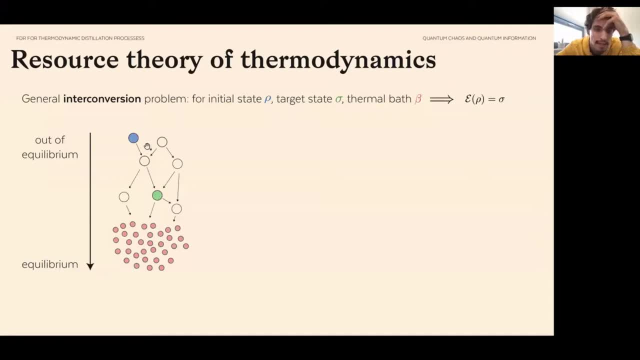 the amount of resource that the state green has is less than the amount of resource that the blue state has. So this is kind of a distillation process And thermal states are in the bottom, because from thermal states you cannot go to anywhere because these states don't possess any kind of resource. 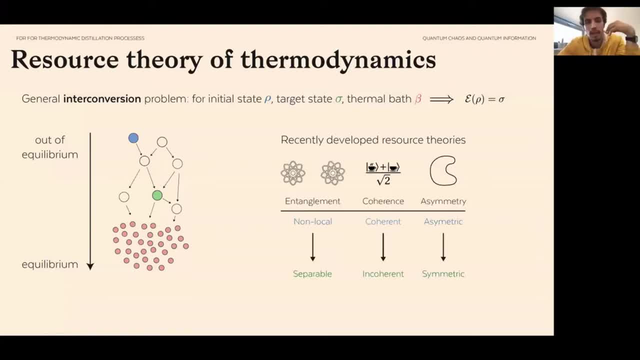 Let me fair and tell you that this is not a unique problem in research here of thermodynamics. But you can ask the same questions in different ways. You can ask the same questions in different resource theories, So for example in resource theories of entanglement in which the set of free objects is all the 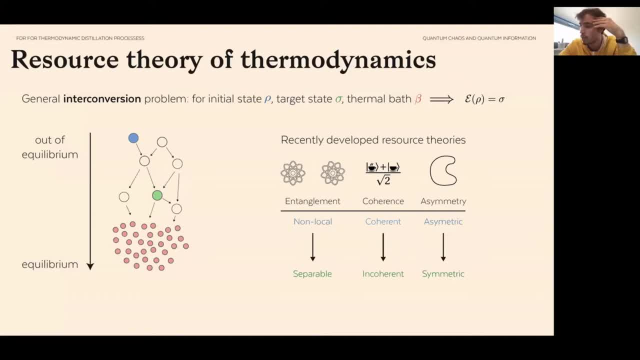 separable states, the set of operations are local operations and classical communications, And you can ask the same questions. Or, for example, in the resource theory of coherence, in which the set of free objects are all in coherent states with respect to some basis. 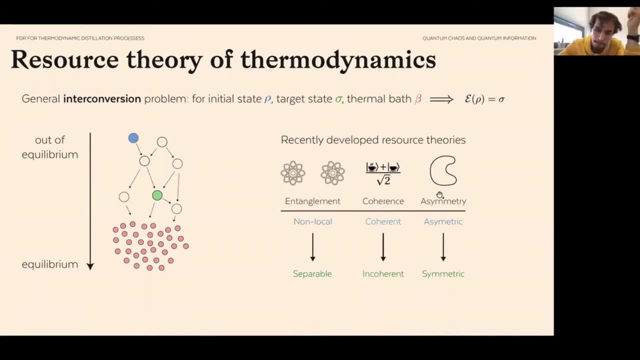 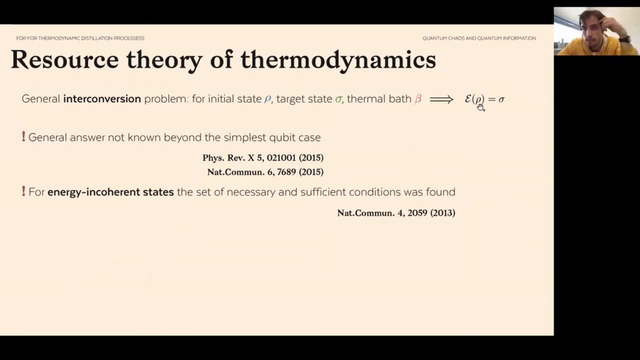 And In the resource theory of asymmetry. Well, so this is the question that we are trying to attack: whether there exists some thermal operation map relative to sigma. But let me tell you that the general answer for this question is not known beyond the simplest case. 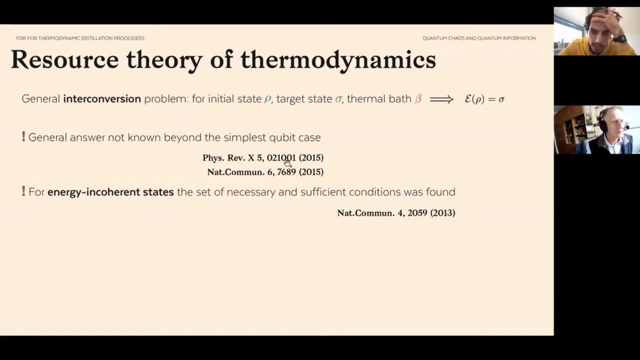 as it was pointed out in 2015 by Camille and collaborators, Although the set of necessary and sufficient conditions was found in 2013 in this paper by Michal and collaborators, for a set of states, which is the energy incoherent states. 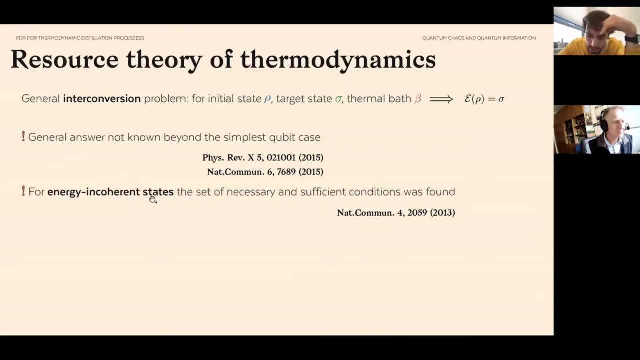 What does it mean to be energy incoherent states? It means that the initial system and the target system commutes with the Hamiltonian of the system And if they commute with the Hamiltonian of the system, they are diagonal in this energy basis. 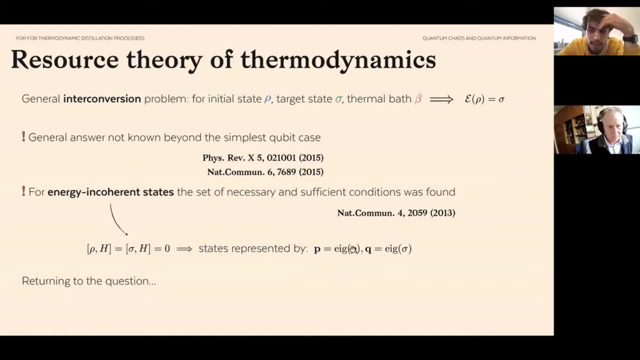 So I can represent these states by probability vectors, such that they are the values of rho and values of rho and sigma respectively, And there exists a thermal operation mapping rho to sigma If, and only if, the thermal majorizes Q. I don't want to give you too much details about what the thermal majorizes means. 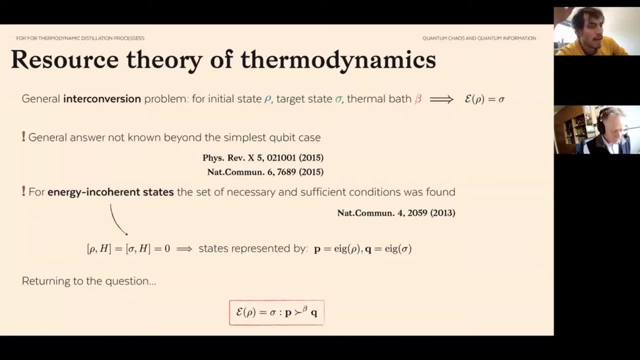 but you can imagine that thermal majorization is a variant of the concept of majorization. So for example in the In the limit in which the temperature tends to infinity, This concept here, that in the limit in which the temperature tends to infinity, 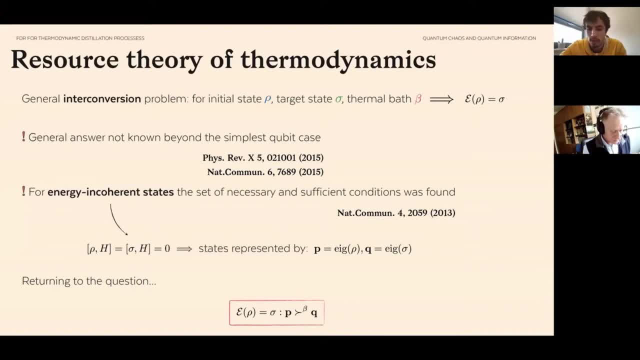 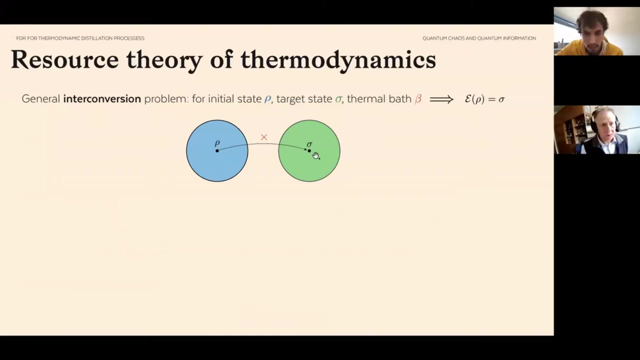 the thermal majorization reduce the case of majorization. Let's imagine the following scenario: Let's imagine that I have my system, rho, and some target state sigma, but I cannot achieve sigma Via thermal operation. This operation is forbidden. I cannot achieve sigma. 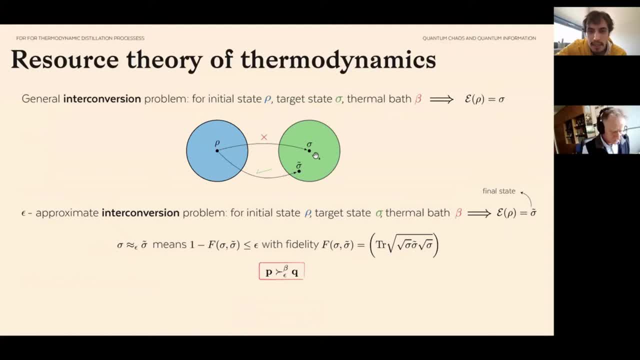 But let's imagine that there exists some sigma tilde in which I can achieve- And sigma tilde is very, very close to sigma in terms of infidelity distance. So in this case we say that this is epsilon approximated interconversion problem. 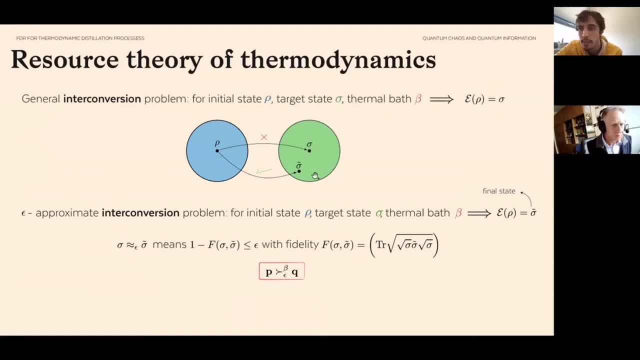 Because you can go to some state which is epsilon away from this state That you want to achieve in with this in terms of infidelity distance. Okay, And we denote usually this transformation like this: P epsilon thermal majorizes Q. Okay, Where this epsilon is the error of the transformation. 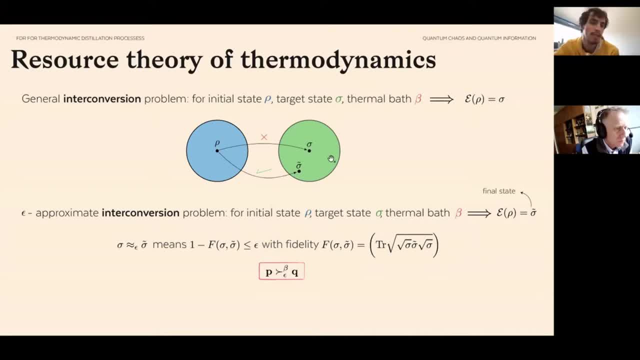 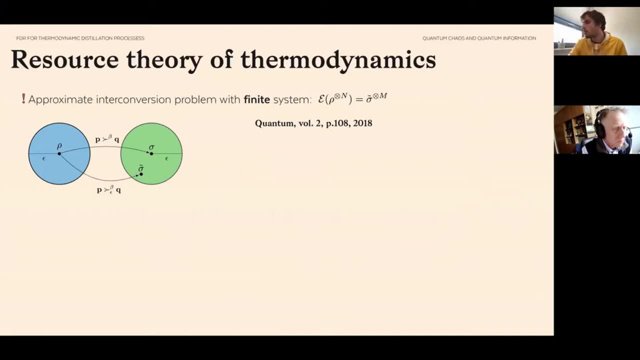 In other words, we can say that we can go from from sigma up to some error. We can. We can always make this problem more interesting because so far I'm telling you about, Let's say, I have a single system and I'm going to another single system. 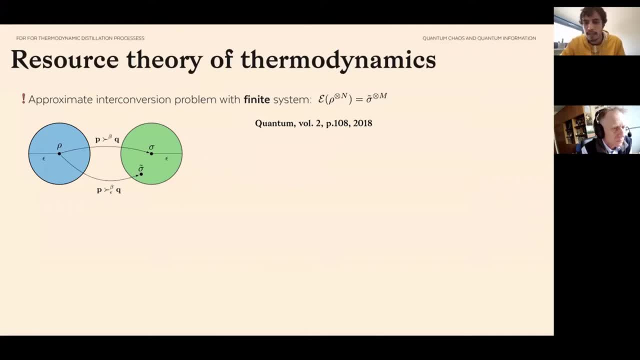 But we can ask how about we have a finite, a finite copies of a given system, So for example, any copies of rho. And then we ask whether we can achieve rho- Sorry, whether we can go, whether we can achieve sigma. Many caught any copies of the state sigma. 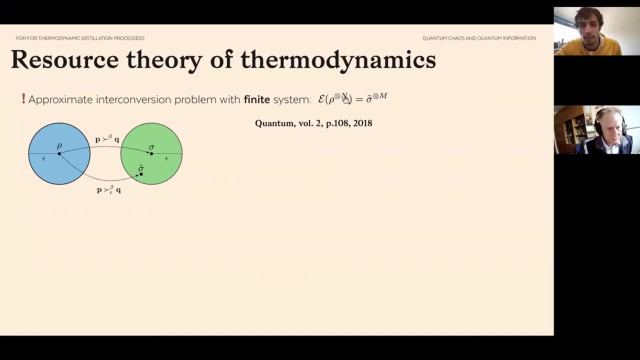 Via any copies of of rho via thermal operation. So this problem was a study in 2008 by a chameleon collaborators And they gave second order rate for energy and coherent state. What does it mean this? It means how many states you can achieve. 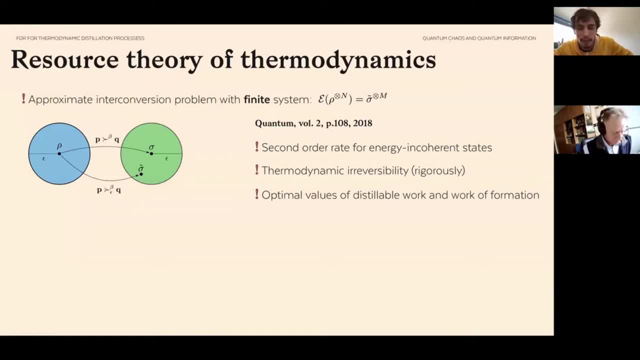 When you restricted this interconversion problem between energy eigenstates. And they study also very rigorously The problem of irreversibility of the state sigma. Okay, So the problem of irreversibility, which means let's imagine that we go from rho to sigma. 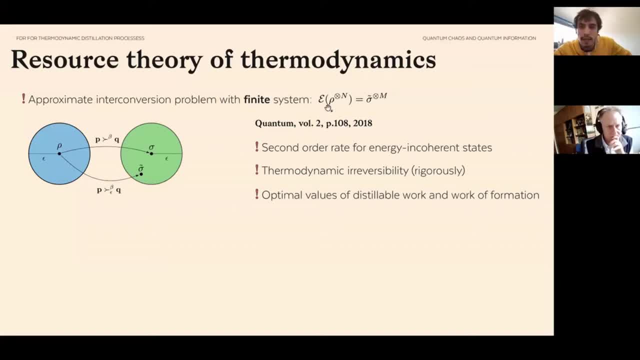 Whether is it possible to return to sigma again. And also they calculated the optimal values for the distillable work, The work that you can extract from a given system, and the work of formation, The work that is required to create some system. However, some questions reminded. 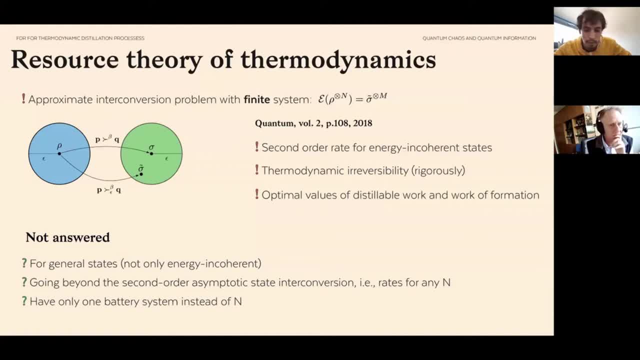 So, for example, They study The interconversion problem between energy and coherent states. And how about for general states? So, for example, how about for general peer states When your initial state is a general peer state, And is it possible to go beyond the second order asymptotic state interconversion? 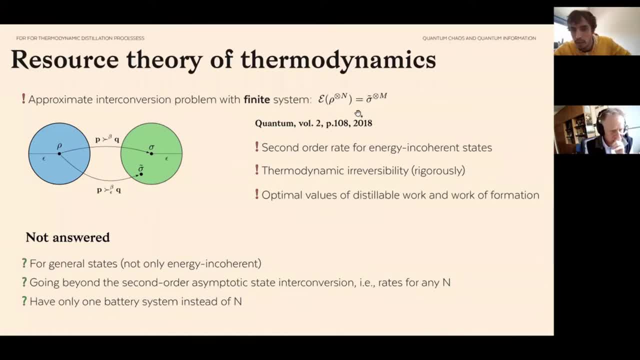 Why? Because the results holds when n tends to infinity And n has to be large. And what if I don't want to look for any large? for example, What is the optimal error of this transformation when I'm working, let's say, with five copies? 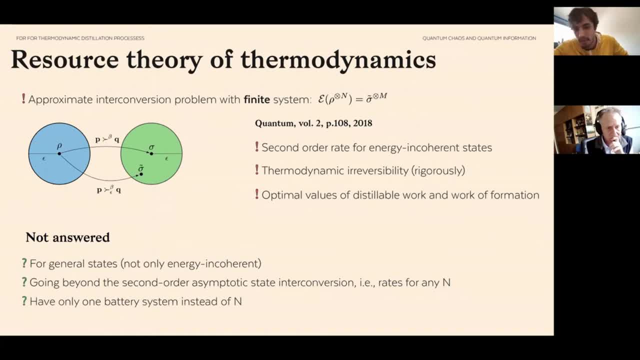 When n is equal to four or n is equal to seven, And also, although I didn't show you, but I'm going to show in the applications. There's a problem in quantum thermodynamics which is very tricky, Which is how to define work. 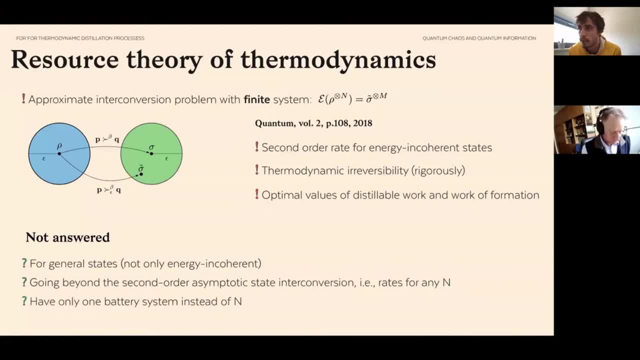 But with the resource framework we can easily define work. I would say, But when you have. But when you have finite copies of a given system to define work, it's a little bit tricky Because work for us, as we see, is usually defined in terms of a battery system. 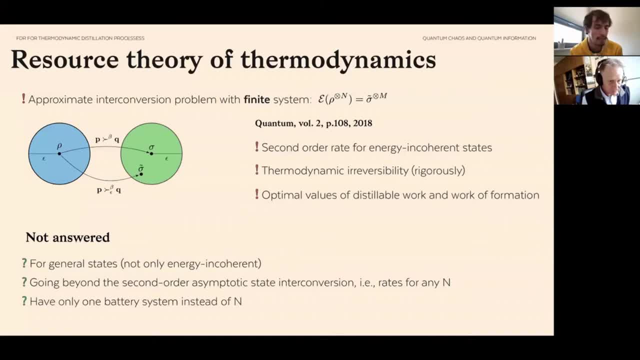 And when you have any cops of a given system. this means that, according to this framework, you need any battery systems, But that it's a little bit difficult to interpret when you have any battery systems Because, as I said, you have some error, you have some fidelity of the battery. 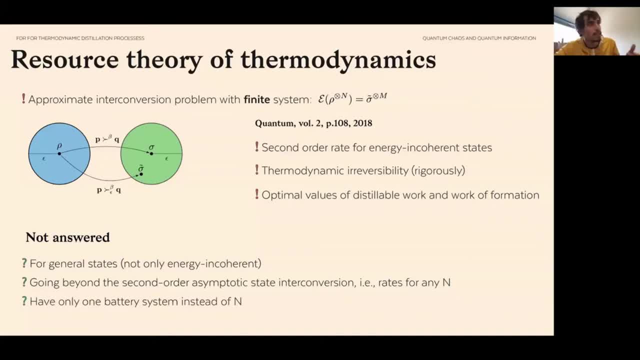 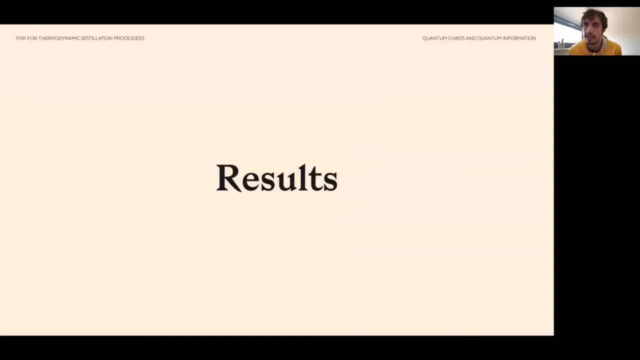 And it's difficult to try to understand what is this fidelity when you have any cops of a battery system. Okay, So that was one of the questions that remained open. So, okay, I think now it's clear. Okay, It's a good time to stop a little bit and see if you have any questions so far about the framework. 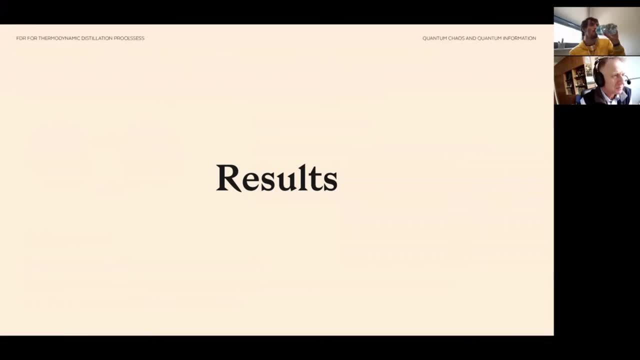 So are there any questions to Alex? I went a little bit fast in this first part about the resource theory framework, But if you have any questions, please you can ask. It looks like it's not the case. I have one. 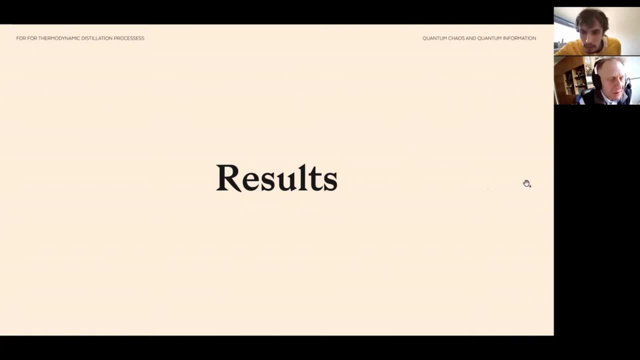 Yes, So there are some. Yes, please, Who's speaking? Fereshteh? Ah, Fereshteh, Hello, Go ahead. Okay, I want to know if satisfying the commutator between local Hamiltonian and the joint unitary operator is also necessary for the map E to have actually invariant state gamma. 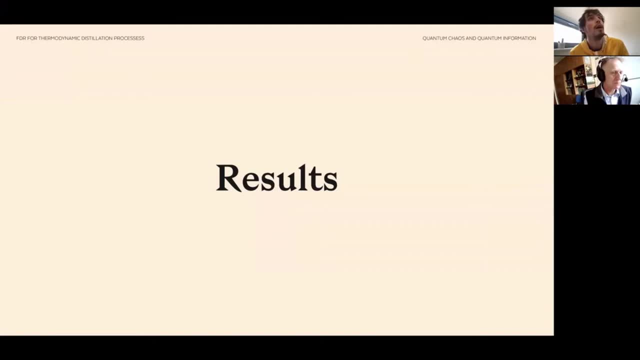 Yes, Necessarily Yes. The condition that we know so far is that the initial system and the targets- the initial state and the target state, must commute with the Hamiltonian of the system. They are diagonal in the energy basis And the unit. 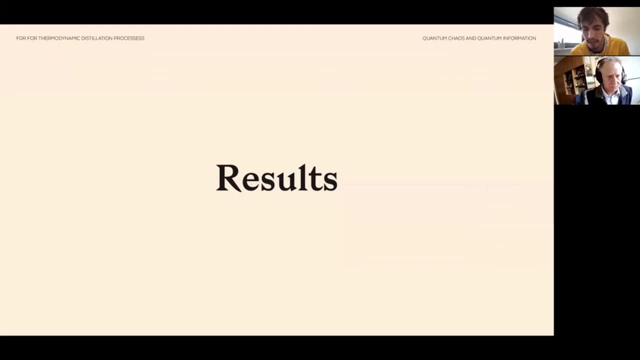 Yes, And the unitary, the energy preserving unitary, must commute with the total Hamiltonian as well. Yeah, If the commutator satisfies, then we get a quantum channel with gamma as invariant state. But I want to know if inverse is true. 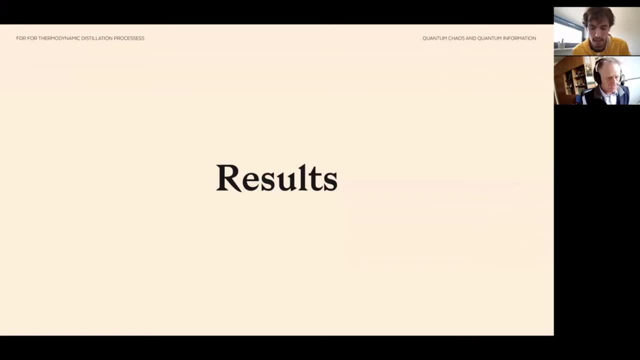 For having a quantum channel with invariant state gamma, then we should have a joint unitary operator that commute- sorry, that commutes with Hamiltonian. Can I just jump in quickly? Yes, please, It's a more general. it's a more general family that you're asking for. 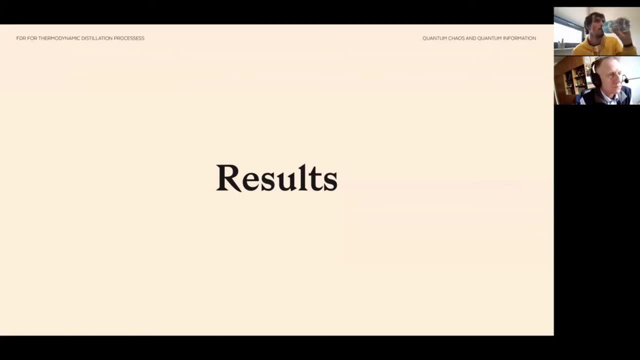 Like, just knowing that the Gibbs state is preserved does not mean that the unitary has to conserve energy. There are other maps that are Gibbs preserving so that they have the Gibbs state as a fixed point, but they can't be realized as the thermal operations here. 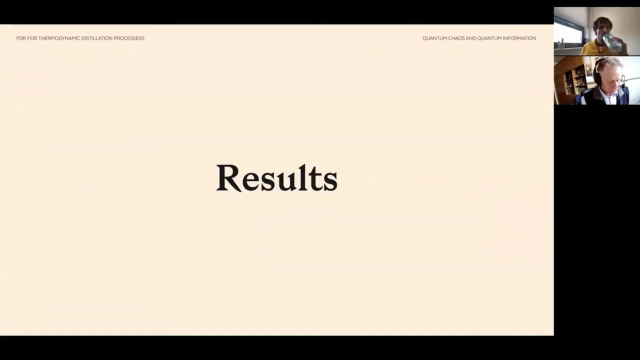 Okay, So we add other restrictions to have those, those of thermal dynamics? huh, Yes, exactly This time. translation symmetry especially. yes, Yeah, Thank you very much, Thanks, Thanks for the question. And okay, So, before I present you the two theorems, our two results, I would like to summarize what, the questions, the questions that we want to answer, and find some quantities which will play a hole here. 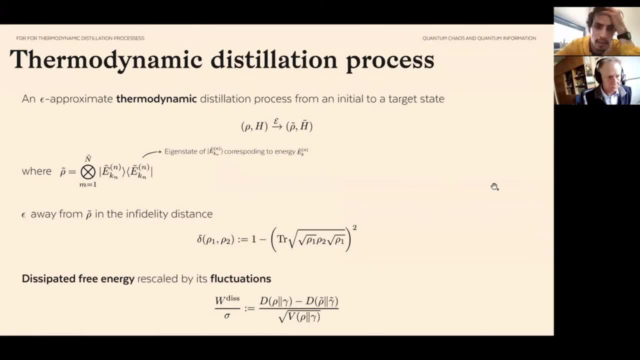 So first let me start by defining what does it means to do: a thermodynamic distillation process. So a thermodynamic distillation process is an approximated thermodynamic distillation process. So the thermodynamic distillation process is the form of a thermodynamic distillation process. 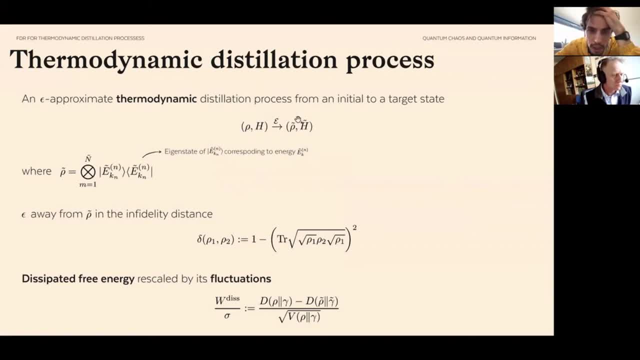 What is it? We start by defining a thermodynamic distillation from a given state row to some energy Eigen state row, to the such that this energy Eigen state- they are given here, where I'm pointing out And and you'll be, uh, it's approximately approximated because we will be epsilon away from the from the from the target state of the final state- is an epsilon only from the from the target. 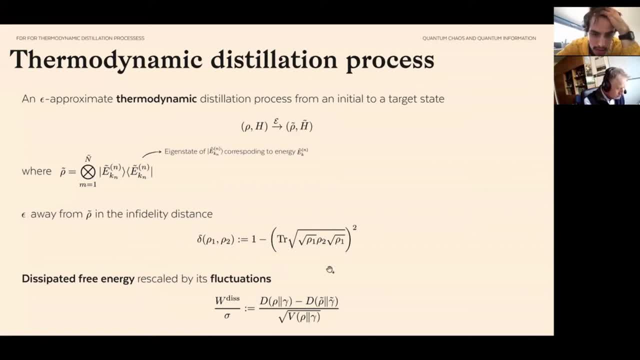 state distance, this distance here, okay, and another so to have a really infidelity distance. yes, yes, yes, exactly yes, sorry, it's missing a square root. yes, that's true. thanks, professor, I know this now. and I was saying: and the other quantity that I want to to define here is this: dissipated free energy. we scale, we. 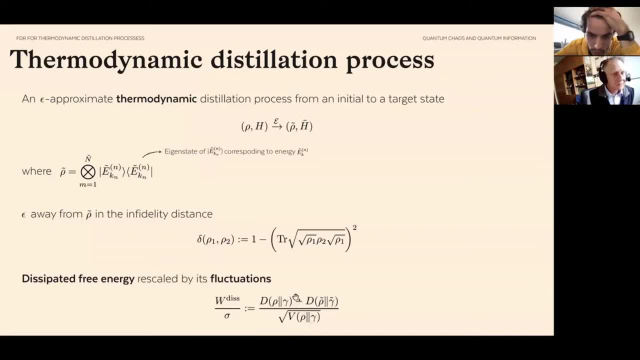 rescaled by fluctuations of the free energy. so, for example, this difference between free energies, here are the work dissipated in this process, the work that you have to pay to go from from a given stage to another. sorry, oh yes, thank you very much. thank you very much, and Sigma here stands for the relative. 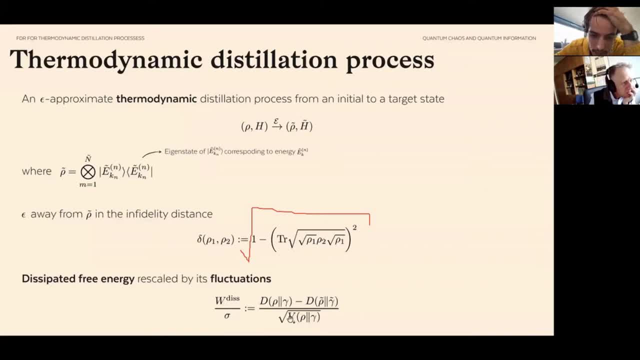 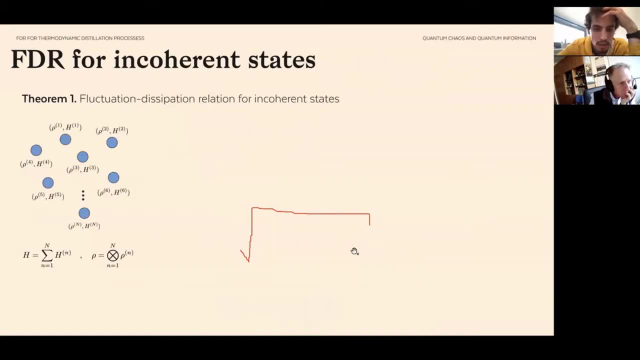 entropy between Rowan and and and gamma and this quantity. here are any free energy fluctuations. okay so, yeah, so basically, let's consider in the following scenario- let's imagine that I have any- I have a composed system consisted by any different subsistence. okay, so, and it so. I have a composite gonna composed by: 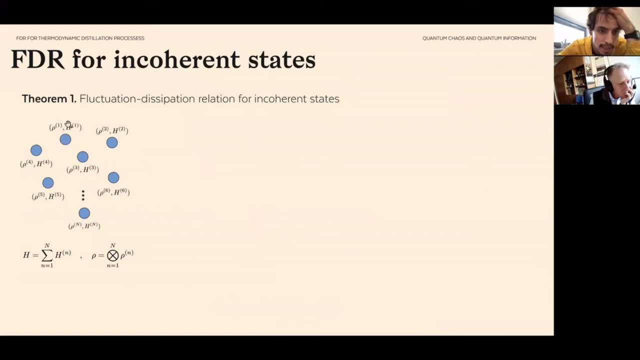 any subsistence, each one described by some state and some Hamiltonian, such that total home. the Tonian, is given by the sum of individual states, and the states are product States, but they are different. okay, so this, this will be my initial state as a target state. I'm gonna have different, different. 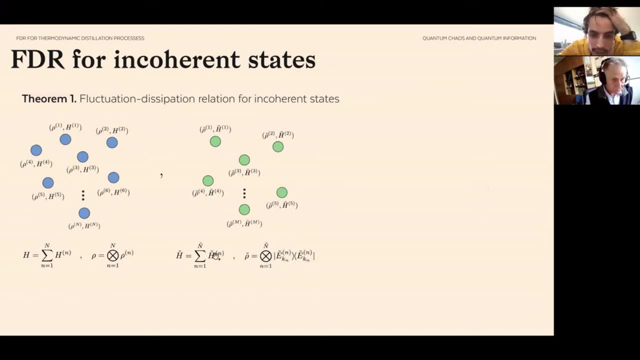 energy eigenstates like these, with different Hamiltonians, and let's imagine that we have any different, any non-interacting subsistence. So my question now, not my question, but our theorem says that there exists a thermal operation mapping this initial state to the target state. 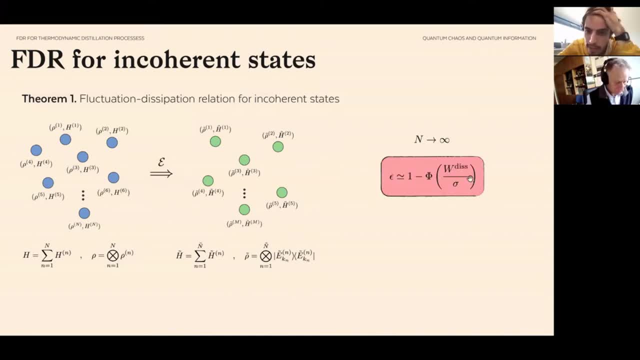 with an error given by this expression when n tends to infinity. So in other words, in the asymptotic limit at which n tends to infinity, the optimal error of this transformation is given by this expression here. Okay, so where phi is the cumulative normal distribution which has this: 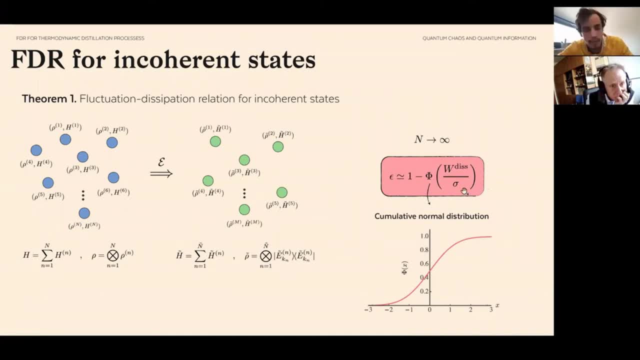 profile here. So basically here- I'm gonna mention this later- but basically here we see that there is a trade-off between the work that is dissipated with the fluctuation. But how about if- and let's imagine that I don't want to look for the 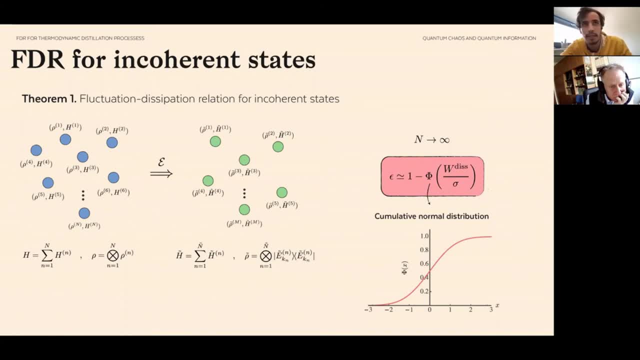 asymptotic limit in which n tends to infinity. but I want to look for a finite n. so, for example, n equal to 5.. In this case there is a thermal operation mapping this initial state to a target state with optimal error. So phi equal to phi. So here the next step is: let's see, let's say we. 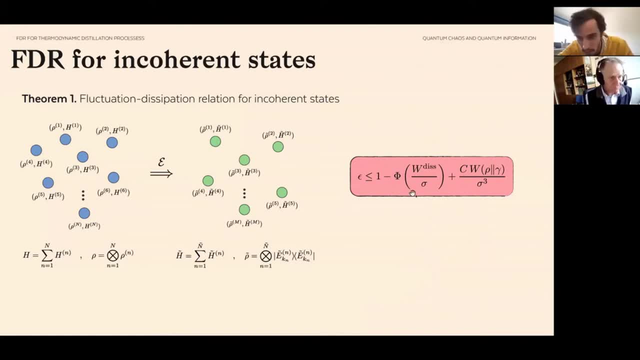 look for an infinite~~. So phi equal to five. So, for example, if phi is an algorithmic function, that and her upper bounded by this quantity here. So again, this phi is the cumulative normal distribution. C is a constant called by a Berry-Essen constant. 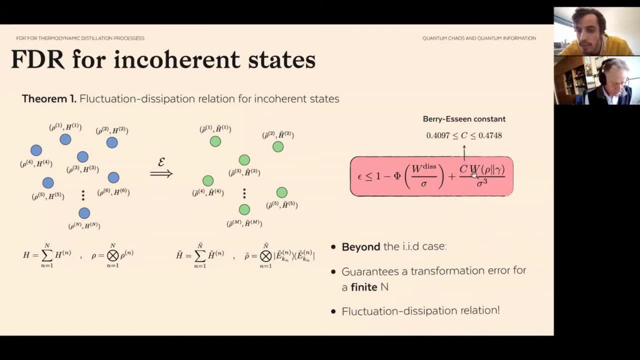 And this W that appears here is the relative entropy skewness which has that interpretation to be thermodynamic interpretation, to be the derivatives of the heat capacity with respect to the temperature when you are measuring between two thermal states with different temperatures. But what I want to emphasize with this theorem one, 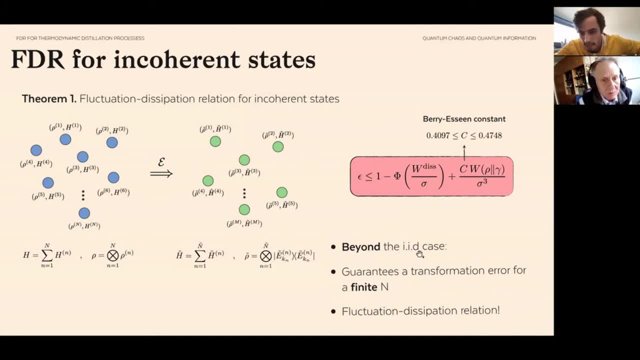 is that we went beyond the IID cases, because here I have any different subsistence, I am not working with copies anymore. Also, that this theorem guarantees a transformation error for a finite n. I don't need to take n to infinity anymore And we see that there's some kind of trade-off. 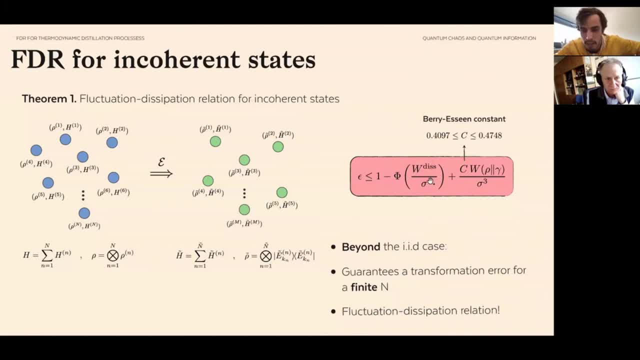 between the work that you do and the work that you dissipated, with the fluctuations, with the free energy fluctuations. In other words, let's imagine that for transformations with the same error but with different fluctuations associated to the initial state, I have different amount of work being dissipated. 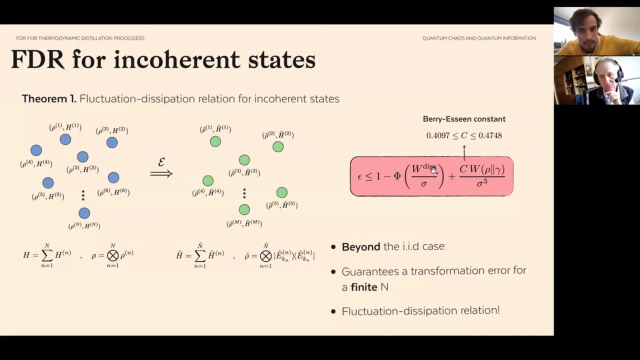 If my initial state has more fluctuations, more work will be dissipated. Conversely, if the initial system has less fluctuations, the amount of work has to be dissipated to achieve the same transformation with this error. This will be more clear when I apply this theorem. 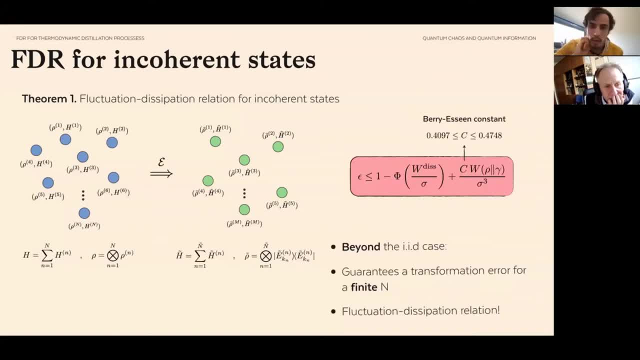 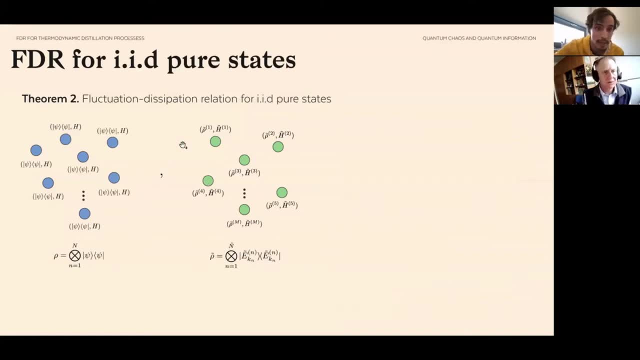 Our second theorem: oh, but let me make a comment here that the initial states they are incoherent states. okay, And our second theorem is for general peer states. But now we have any copies of a general peer states, for example. 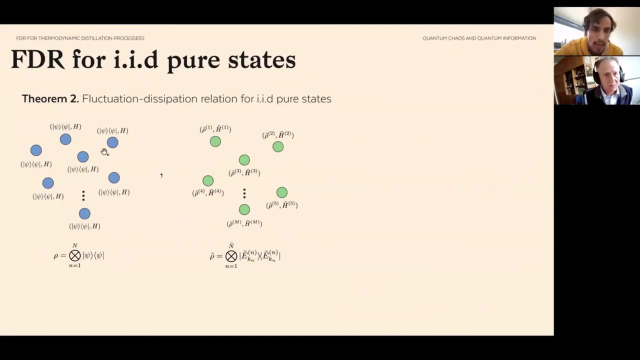 this state here can be the state plus plus, And as a target state I choose some m different subsistence, each one described by some energy eigenstate with its own Hamiltonian. And the theorem too states that there is a thermal operation mapping the initial state. 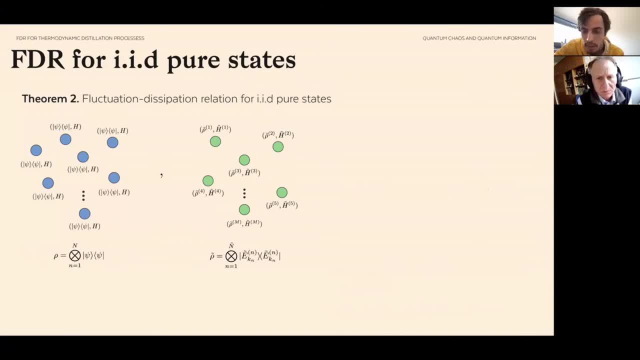 to the target state in the asymptotic limit, in which when n tends to infinity, with an error given by this expression here, as we saw in theorem one. But now let me point it out that we went beyond incoherent states. 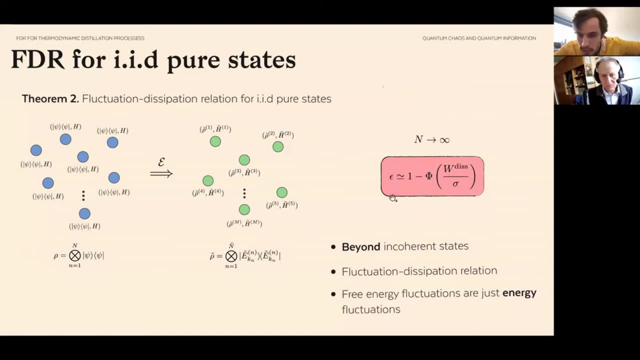 because here I'm dealing with general peer states. Again, we see this behavior between the work that is dissipated with the fluctuations that the initial state have, And also let me mention that these fluctuations here are energy fluctuations because this state is period. 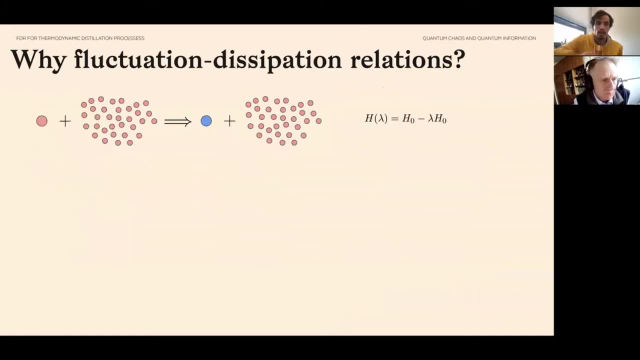 and you can show this. But the natural question is: okay, we see that there is a trade off between the work that is dissipated with the fluctuations associated to the initial state. but why fluctuation-sipation relation? What is a fluctuation-sipation relation? 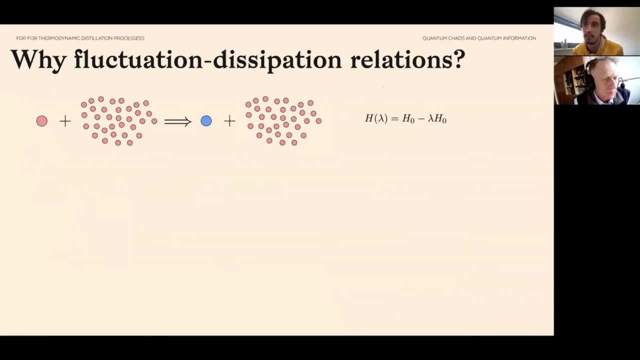 And to answer this question, I would like to connect what I've been talking with a very, very good friend of mine who is a scientist, who has a very nice idea in statistical mechanics. And let's imagine, let me show you this simple problem. 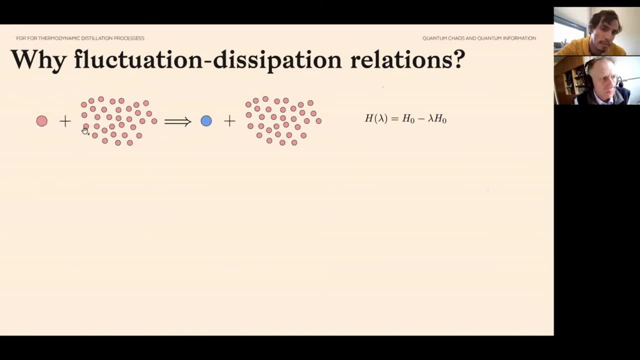 in which I have a thermal system, a thermal state, sorry, I have a system in the thermal state And this system is: there's a bath at inverse temperature. beta, They are in thermal equilibrium And this system is described by some Hamiltonian H zero. 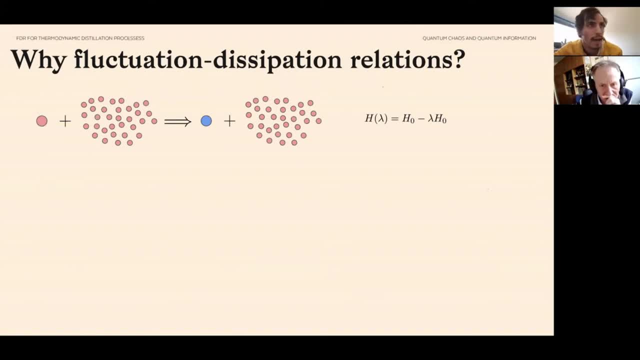 And what I'm gonna do is I'm gonna perturb the system by changing its Hamiltonian and then I'm gonna look to the response of this system after I perturb this system. But I'm gonna do this in a way. 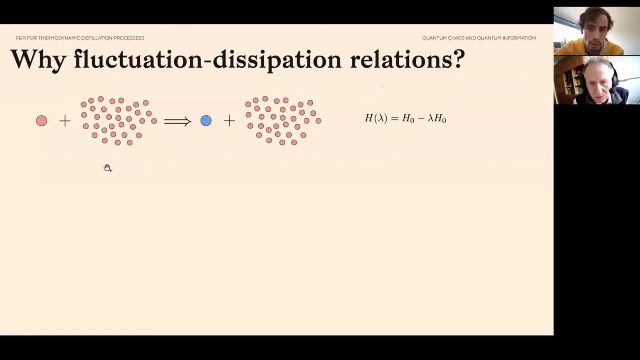 that I'm gonna do a little perturbation in the Hamiltonian. So, for example, I can write the Hamiltonian as a function of this lambda here in this way, And I'm gonna do a little perturbation because I want to use the framework of linear response. 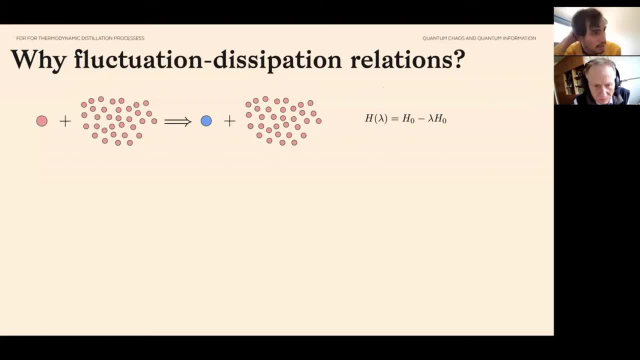 which is a well-known framework from statistical mechanics to see the response of my system. Okay, if I do this, I will get that the dissipated work. the dissipated work is proportional to the energy fluctuations that the system have when the system is in thermal equilibrium. here, 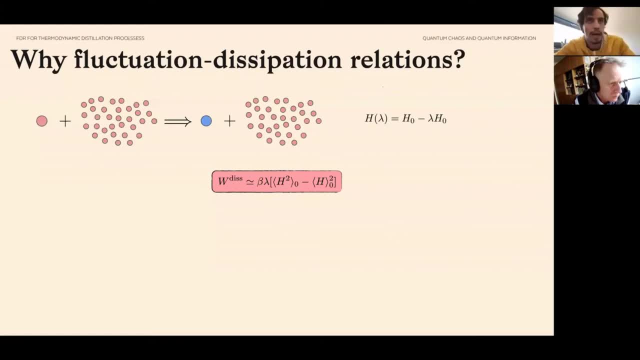 So basically, this can be very well captured by if we remember about the Brownian motion. Let's imagine that we have a particle and this particle is immersed in some liquid and this particle is immersed in some liquid and this particle is immersed in some liquid. 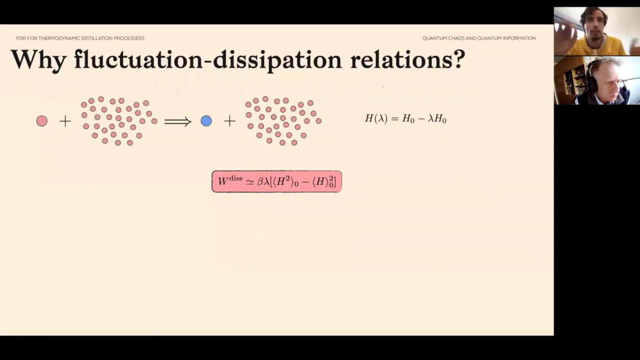 and this particle is jingling because of the thermal fluctuations, And then I push this particle over across this fluid. When I push this particle, this particle will start to collide with the other particles. I'm gonna dissipate it, connect energy. 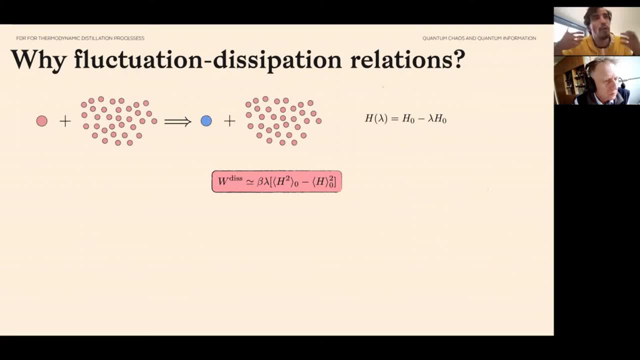 and this dissipation. it's connected with the fluctuations that the particle had when the particle was in equilibrium. Okay, And what our theorem one and two says- is basically a different way to state the theorems- is: let's imagine that we fix some error of the transformation. 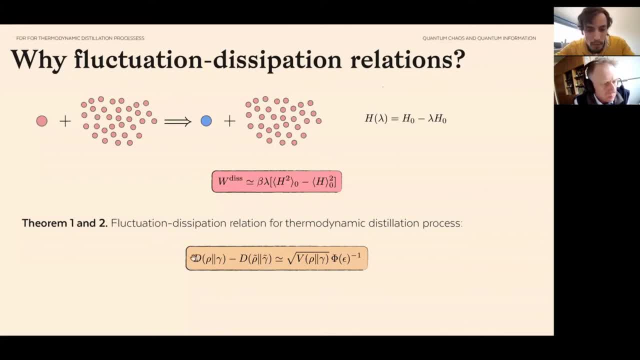 So what our theorem says is that the amount of resource that has been distillated, the amount of work that has been dissipated, is directly connected with free energy fluctuations of the initial system. So we see a big similarity between these two different frameworks. 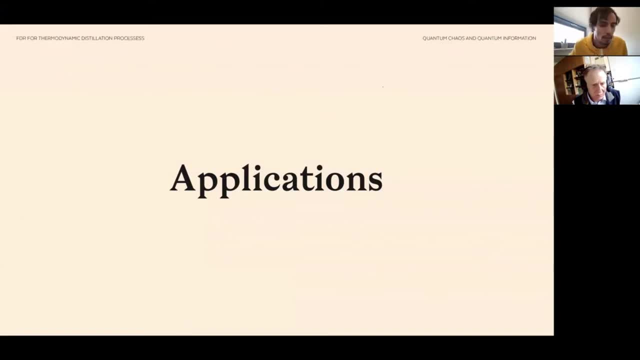 And this is why we call these relations by fluctuation, dissipation relation, because the amount of work that I'm gonna dissipate it it's directly connected with the fluctuations that my system have when my system is, let's say, in the initial state row. 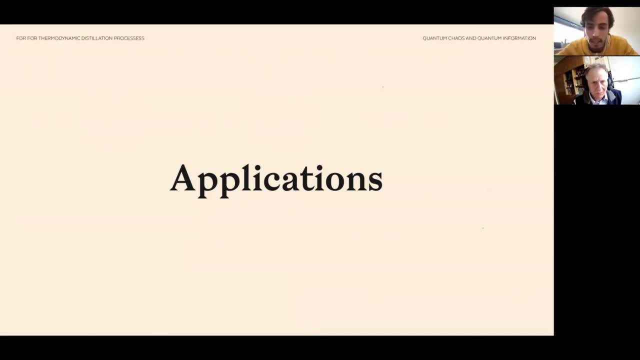 Okay, So let me briefly apply the theorem one and two for two applications. And to do this, in order to do this, I would like to define, to show you how we define work in the resource, theoretically, framework. So let's imagine that initially, my system is composed: 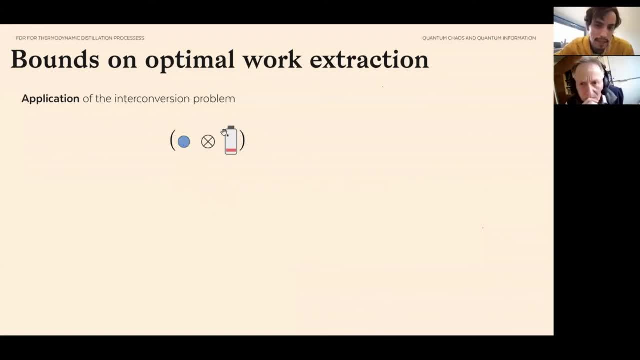 by a given blue ball and a battery system And this battery is empty. This battery is one charge And then I ask whether there exists some thermal operation capable to thermalize the system while charging the system. So let's imagine that I can charge in this battery. 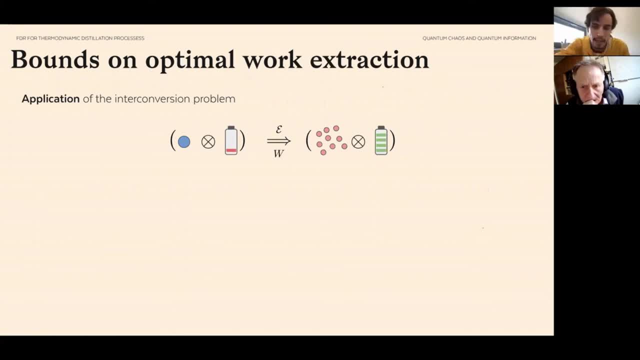 And the cost of this transformation. we define work, The amount of work that I can. let's imagine the amount of work that I can store in this battery system And, for example, I can imagine that this battery is a qubit in the ground state. 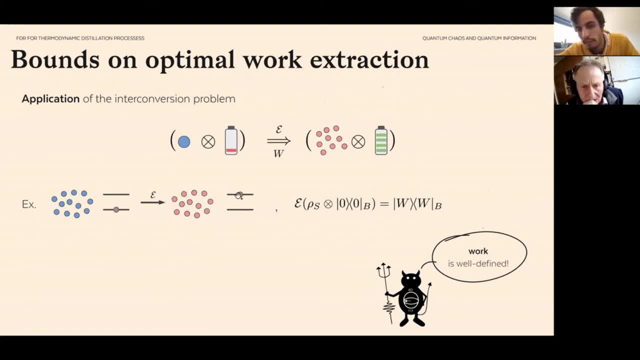 And after the thermal operation, I promote this qubit to the excited state, for example, And mathematically I can represent it like this. So now we see that point that I mentioned about that framework that Kamil introduced in 2018,. 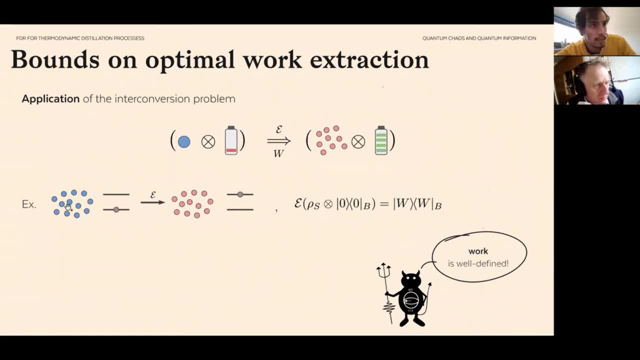 which- let's imagine that you have any cops of your system- You would have, according to that framework, any copies of a battery system again, because that framework was for copies of a given initial system. So now I'm gonna show you how we can correct this. 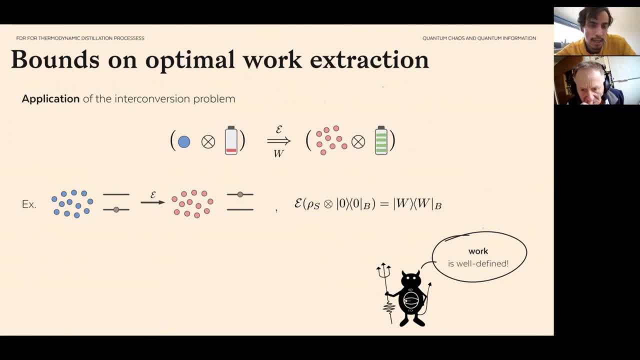 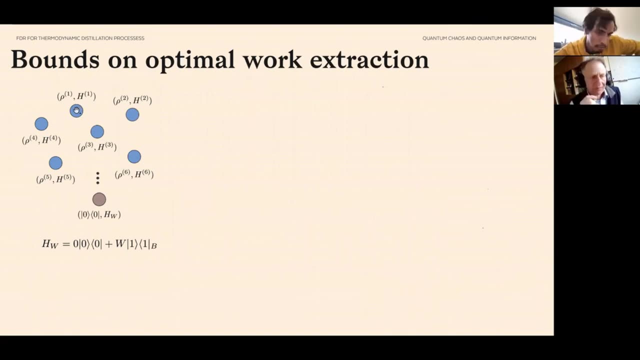 in a way that we have just a single system as a battery system, and how we can extract more information using our theorem about this setting. So let's imagine that I have any non-interacting subsystems, each one different from each other, But the last one I choose to be a battery system. 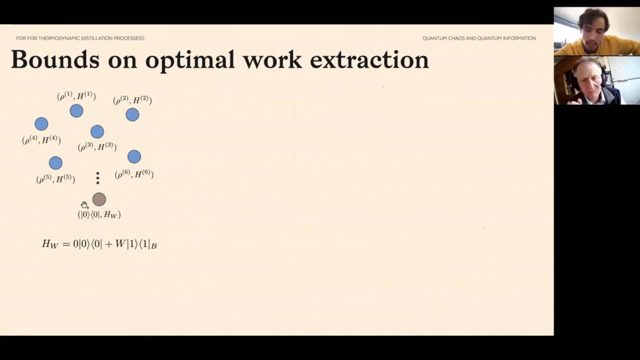 in the ground state with this Hamiltonian here As a target state. I throw away all of the systems. I kept this battery system, but now this battery system in the energy- sorry, in the excited state. So now our theorem says that there is a thermal operation. 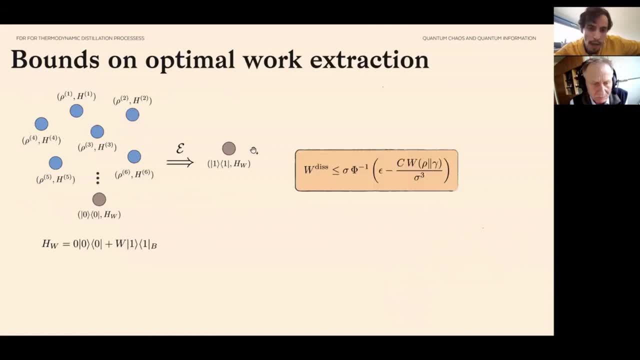 mapping the initial state to the target state, with there is a thermal operation, mapping the initial state to the target state And the work dissipated in this process is given is upper bounded by this quantity here. So, in other words, to make this transition happen. 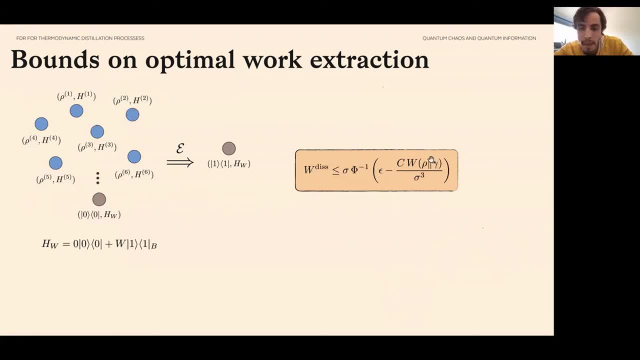 we have to dissipate at least these amount of work, and the work that to dissipated is connected with the fluctuations that the system have in the initial. it's connected with the fluctuations that the system have. Also, our theorem says that the optimal or of this 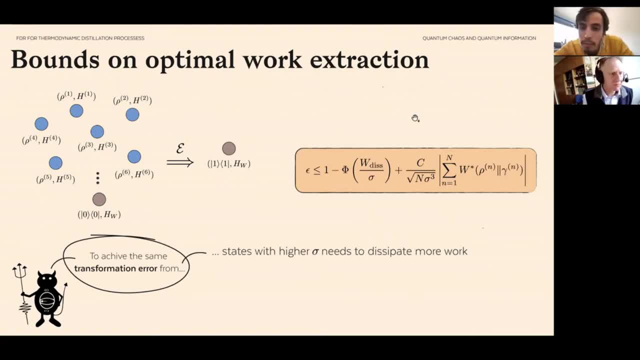 transformation for any end is upper bounded by this quantity. here, And for example, to achieve the same transformation error from system with higher fluctuations, we need to dissipate more work for a fixed error. Conversely, to achieve the same transformation error from states with small fluctuations, 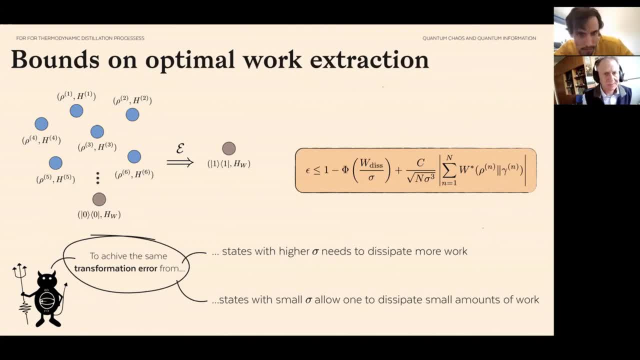 allow us to dissipate small amounts of work. And let me summarize So basically, in this transformation we have to dissipate some amount of work and the dissipation is connected with the fluctuations that the initial system has. Again, the optimal error of the transformation holds. 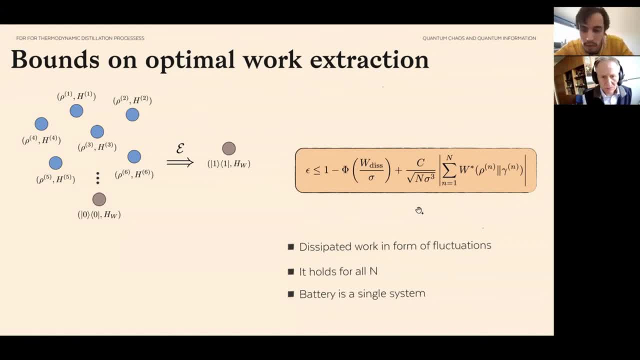 for all n, n can be three or n can be four, And here, with this framework, this theorem, allow us to have only a battery as a single system, like here. We don't need to have any copies of a battery system anymore. The second application: 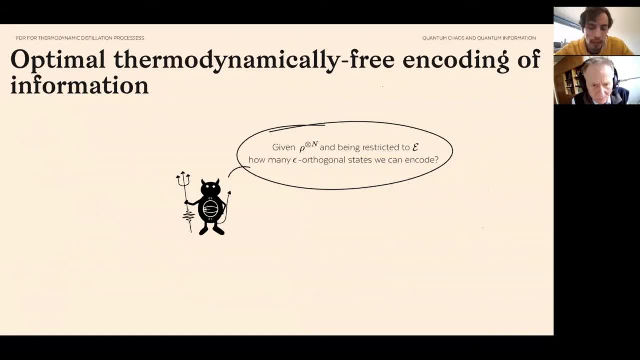 that I wanted to show you is the optimal encoding of information, which can be recast in the following question. Let's imagine that it is given towards some many copies, any copies of a given, of a given system row, And we are restricted to only perform thermal operations. 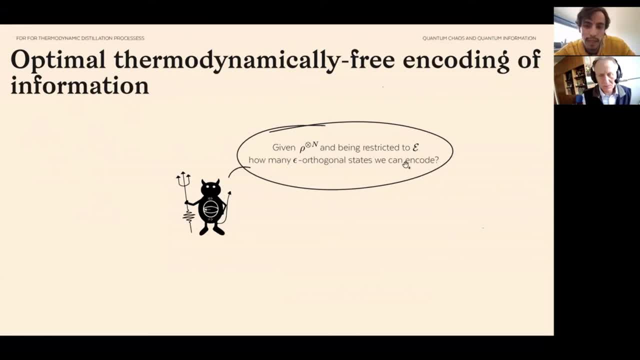 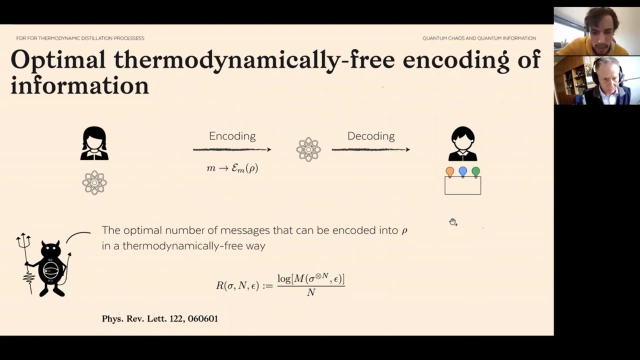 So the question is how many epsilon orthogonal states we can encode into this given system. Epsilon orthogonal because they are all the same. they are orthogonal up to some error. Well, from this paper from 2018, sorry, there's no, the date is not appearing here. 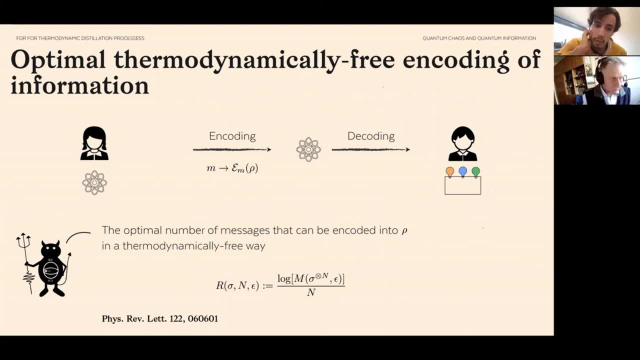 but it's from 2018, it's a paper by Millet-Gou. We know that the optimal number of message that can be encoded into a given system in a thermodynamically freeway- thermodynamically freeway means using thermal operations- is quantified by this quantity here. 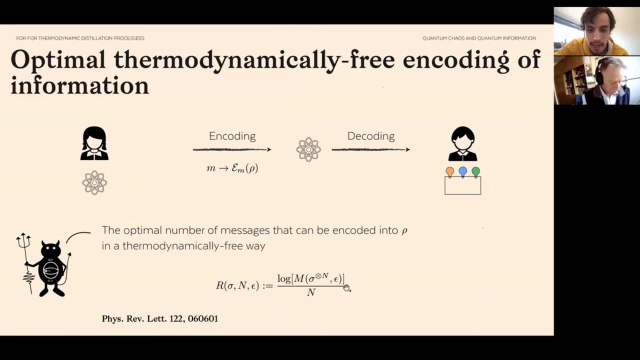 So in this paper they gave an expression for the asymptotic limit, And with our theorem we can give some second order, asymptotic answer for this, such that the first term is the non-equilibrium free energy and the second term is the relative entropy. 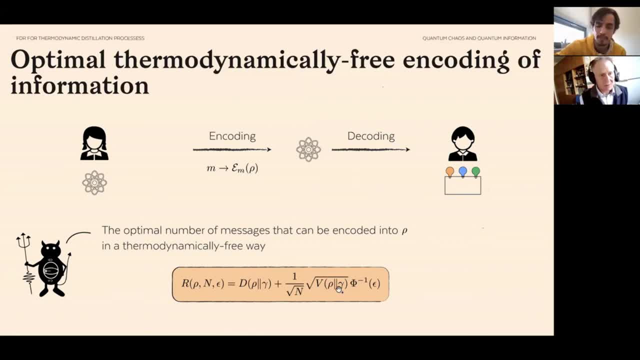 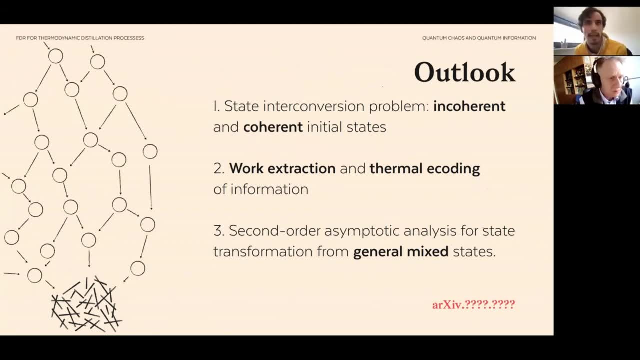 between rho with respect to the thermal state. Okay, so let me summarize about everything that I told you today and we can discuss. So first I show you that the theorem one allow us to work with different subsystems, although they are energy incoherent states. 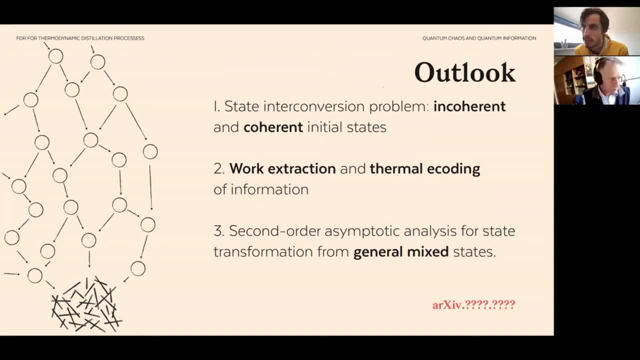 but they are different, with different described by different states and different Hamiltonians, And this is very, very interesting for many reasons because, for example, we can think, in modeling a gas, for example, using this framework, of course, that this is an optimistic thought. 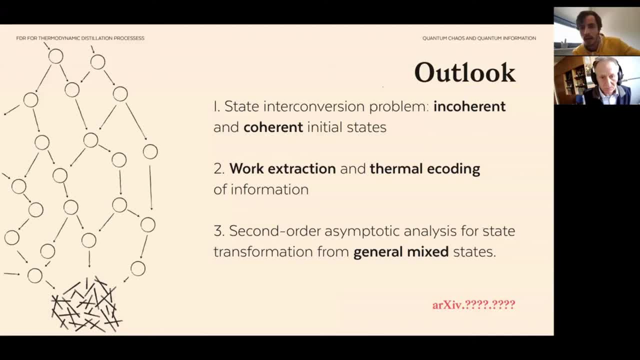 but we are evolving towards this direction. I also showed to you that we went beyond the incoherent states by considering general pure states, many copies of general pure states, into energy eigenstates. And then I apply it very briefly, our results for the problem of work extraction. 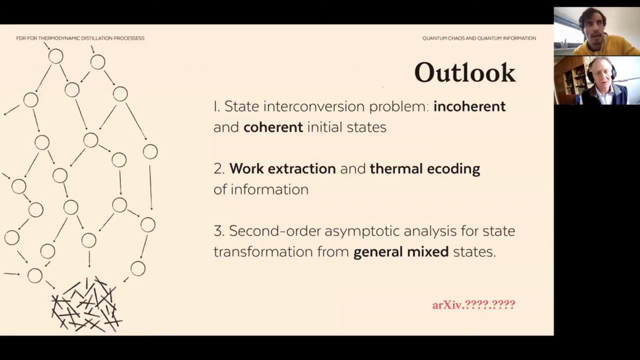 and the thermal encoding of information, And I would like to finish my seminar by with a question, which is: and how about for general mixed states? Is it possible to do this? And this is one of the questions that we are working on And, yes, I hope we got it for next time. 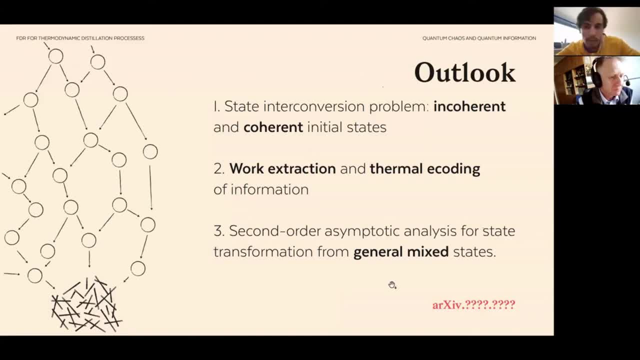 I present to you again. So this: if you are interested in this work, this work will appear on our archive, maybe next month, and it's that So oops, Oh, I forgot it, Thank you. Thank you very much. 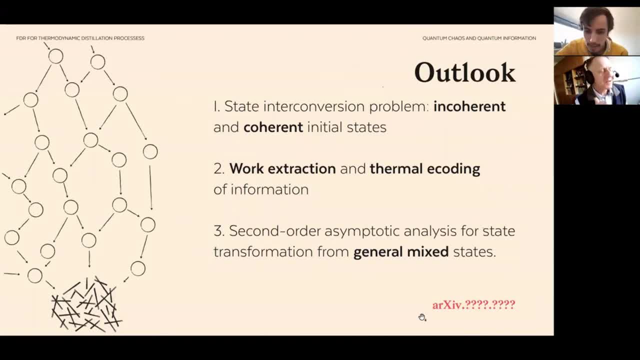 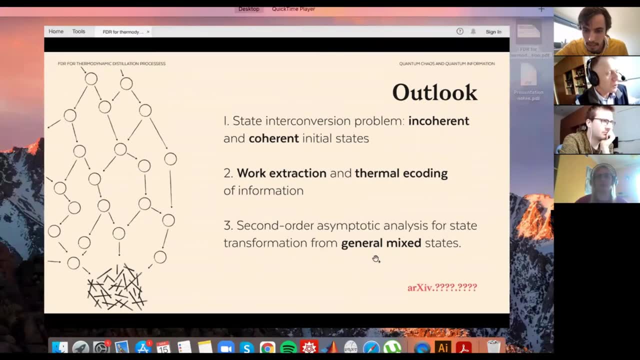 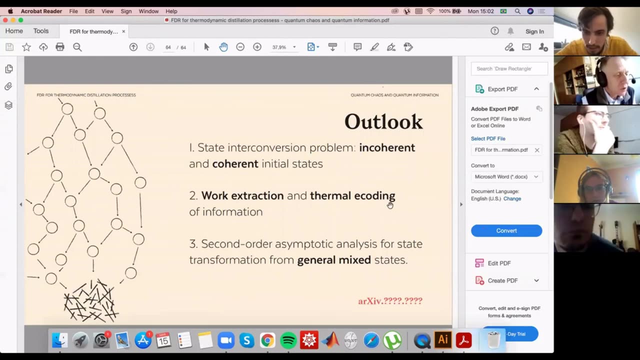 Yes, Thank you very much. Thank you, Alex. Thank you for a very nice talk and for yes, ahead of schedule, So I it was not necessary to issue you any helpful warning. It's perfect. okay, Let us start now the discussion. 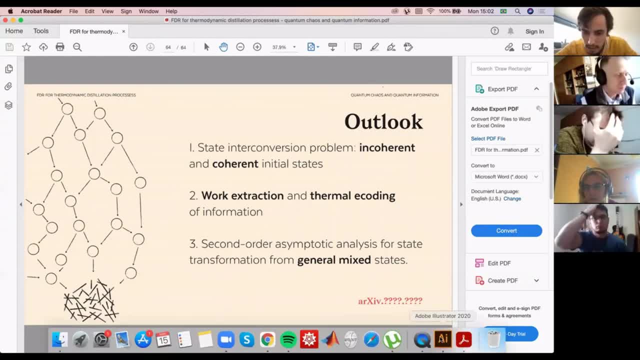 Who would like to make a comment or ask a question, Please? Oh, you can also write by chat.